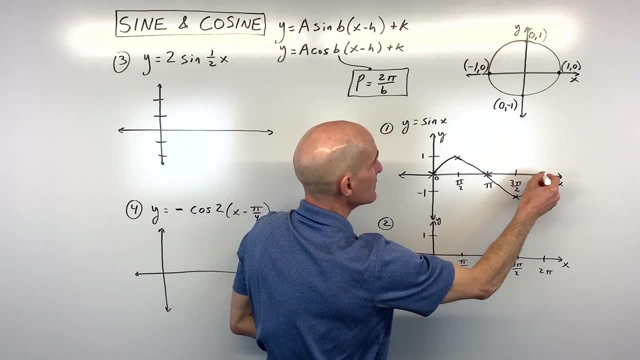 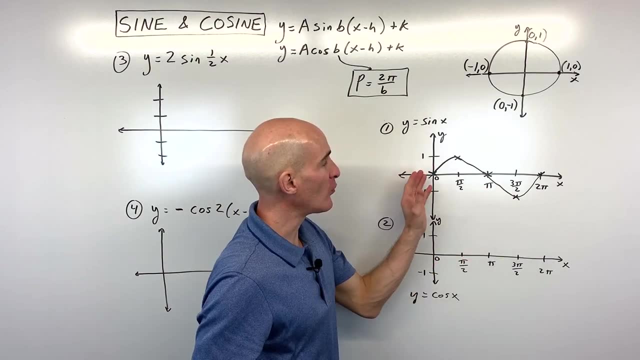 is that this graph just repeats like this- It's like an s shape, forever and ever. So it's good to have a basic understanding and kind of a memorization of what the basic shape of the sine graph looks like. What I like to think of is it starts at the midline. it 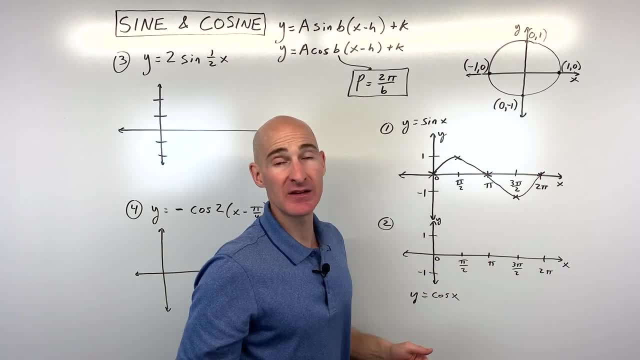 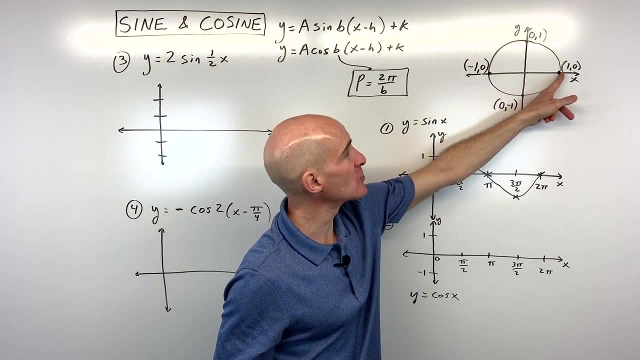 goes to the maximum, back to the midline, minimum, back to the midline. Now let's look at cosine. Same idea: when you work with cosine, you're going to look at the x coordinates. okay, So cosine of 0 radians is going to be 1, so we actually start. 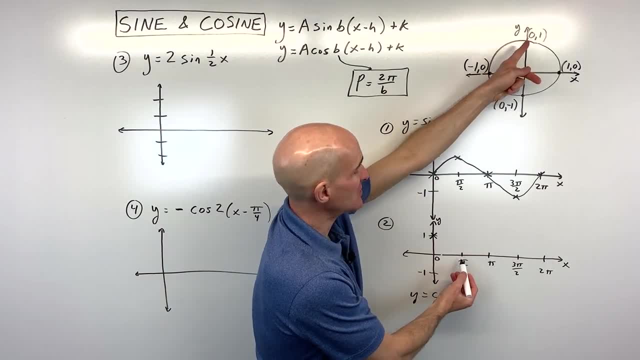 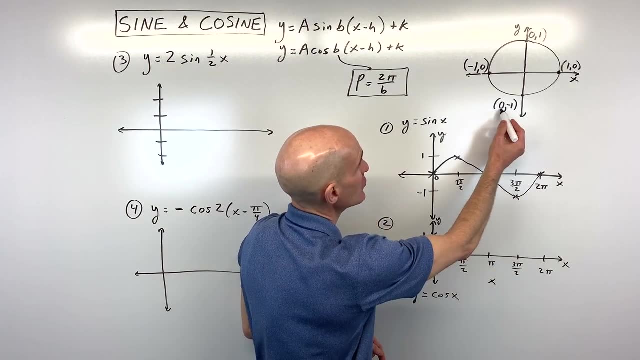 up here: at 1. At pi over 2 or 90, you can see that cosine is going to be 0.. At pi, you can see that cosine is negative. 1. At 3 pi over 2, cosine is going to be 0, and at 2 pi you're. 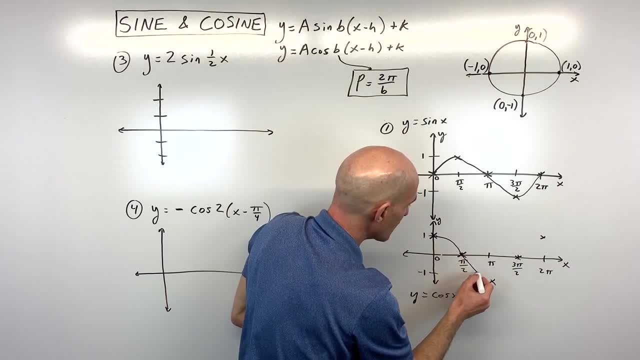 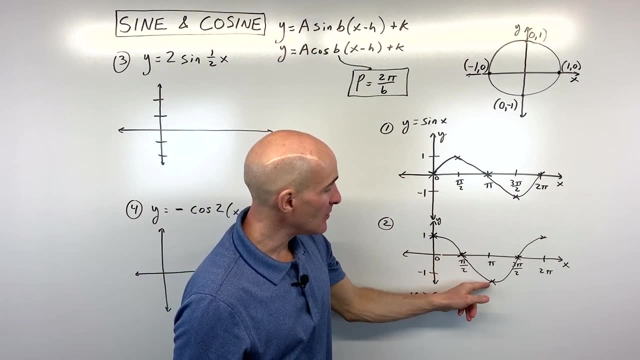 back to 1.. And so you can see. the basic shape of the cosine graph looks something like that, And I like to think of it as starting at the midline, Starting at the maximum, then going to the midline minimum, midline back to the maximum. 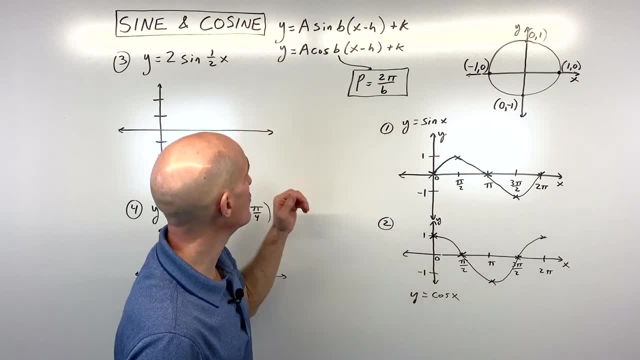 So, again, you want to memorize the basic shape for cosine. It'll make it easier when we go into these more challenging examples that we're going to be doing next. So first let's start off with kind of a basic one, and then we'll get more challenging as 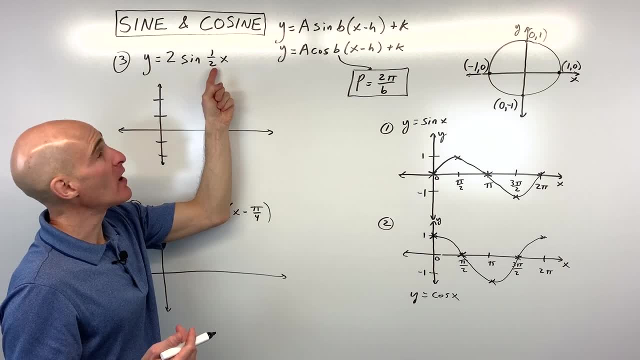 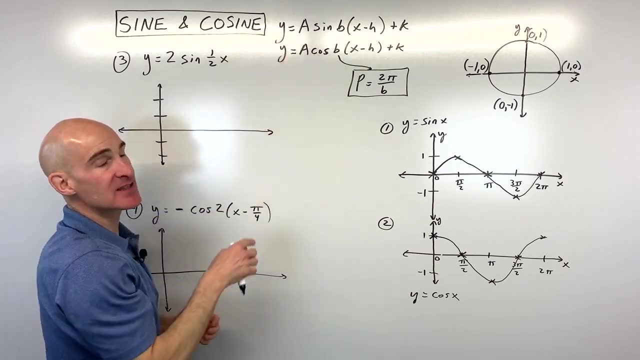 we go See if you can graph: y equals 2 sine 1 half x. Okay, so the way I would approach this is I would say: okay, this number that comes in front of the sine or the cosine that's involved with the vertical stretch or shrink, If it's greater than 1, it's going. 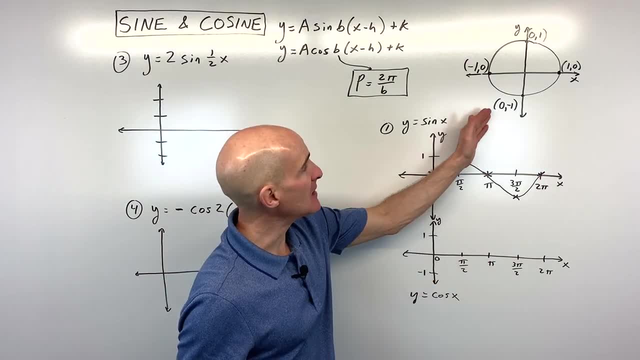 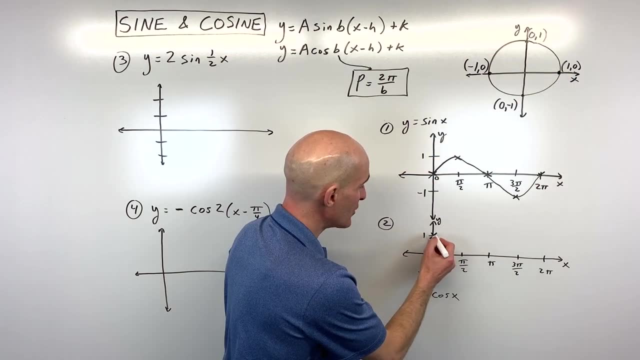 back to the midline. Let's look at cosine. Same idea: When you work with cosine, you're going to look at the x coordinates. So cosine of zero radians is going to be 1.. So we actually start up here at 1. At pi. 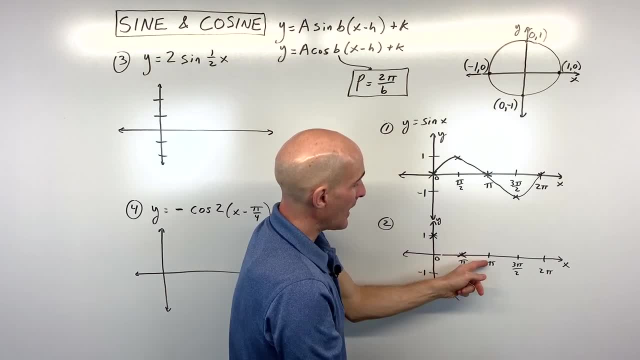 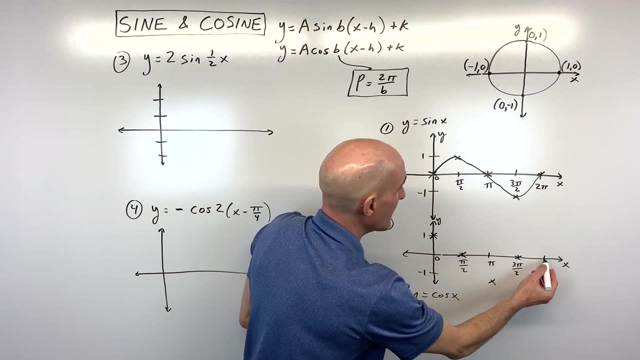 over 2 or 90, you can see that cosine is going to be zero. At pi, you can see that cosine is negative: 1.. At 3 pi over 2, cosine is going to be zero, And at 2 pi you're back to 1.. And so you can see the 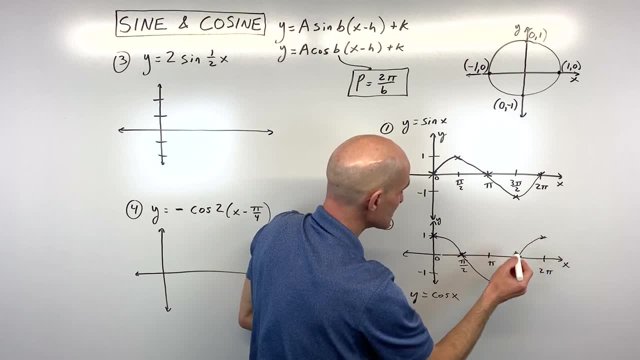 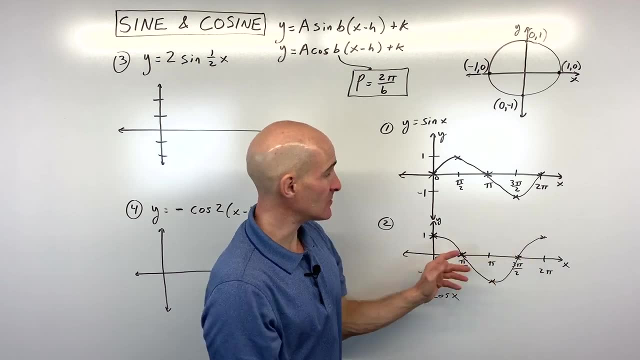 basic shape of the cosine graph looks something like that And I like to think of it as starting at the maximum, then going to the midline, minimum midline, back to the maximum. So again, you want to memorize the basic shape for cosine. It'll make it easier when we go into these. 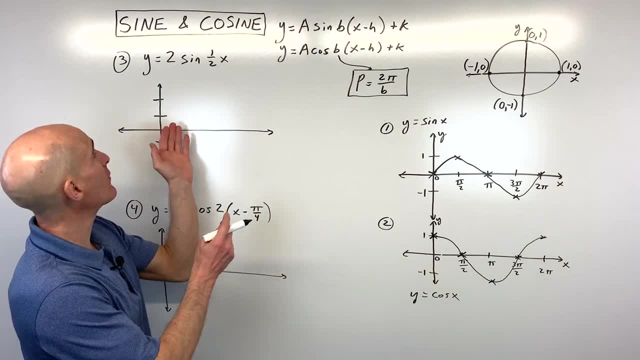 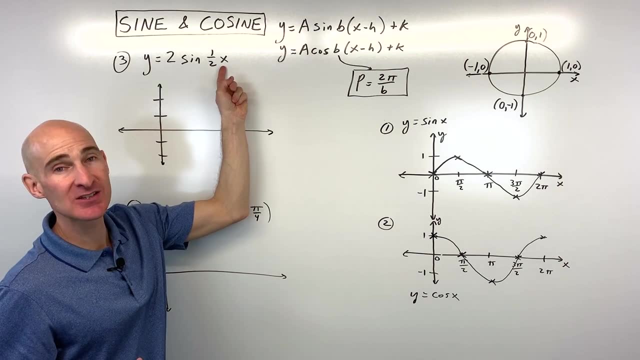 more challenging examples that we're going to be doing next. So first let's start off with kind of a basic one and then we'll get more challenging as we go. See if you can. graph y equals 2 sine 1 half x. Okay, so the way I would approach, 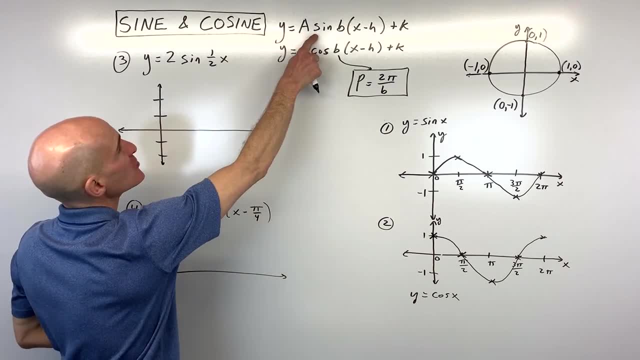 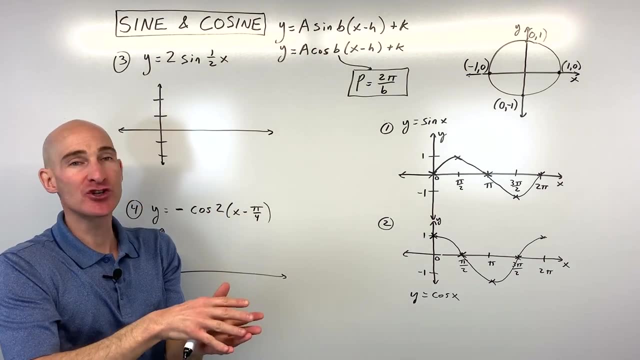 this is, I would say, okay, this number that comes in front of the sine or the cosine that's involved with the vertical stretch or shrink. If it's greater than 1, it's going to be a stretch. If it's between 0 and 1, it's going to be a shrink. This is what we. 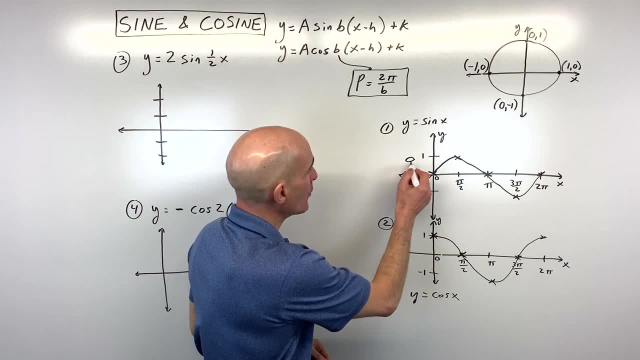 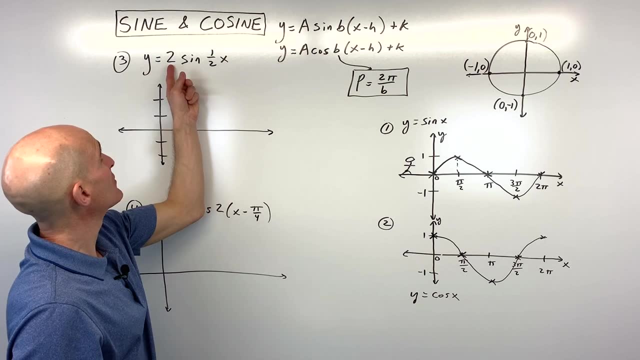 call our amplitude, And when you think of amplitude, you can think of these as like waves, And it's like: how high are the waves from that midline? Okay, And so what you can do here is you can see that they're going to be too high. Okay, And so what's going? 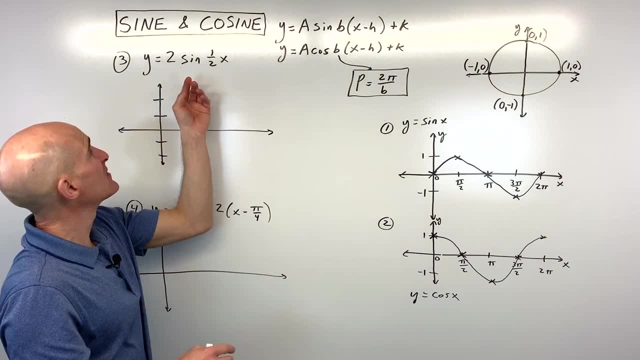 to be a stretch. If it's between 0 and 1, it's going to be a shrink. This is what we call our amplitude, And when you think of amplitude, you can think of these as like waves, And it's like how. 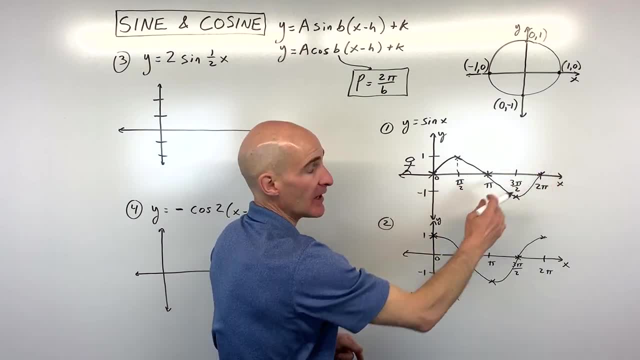 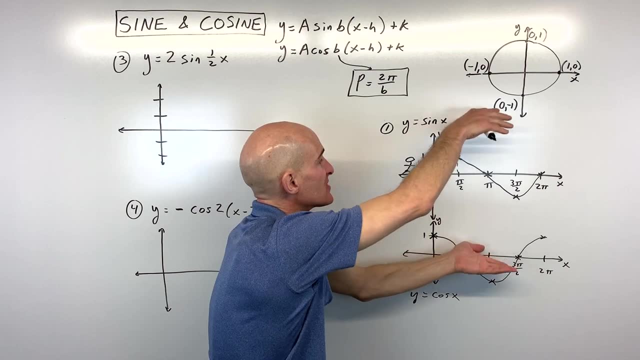 high are the waves from that midline? Okay, and so what you can do here is you can see that they're going to be too high. Okay, and so what's going to happen is it's going to be a vertical stretch of the sine graph by 2.. Okay, you're multiplying all the y values. 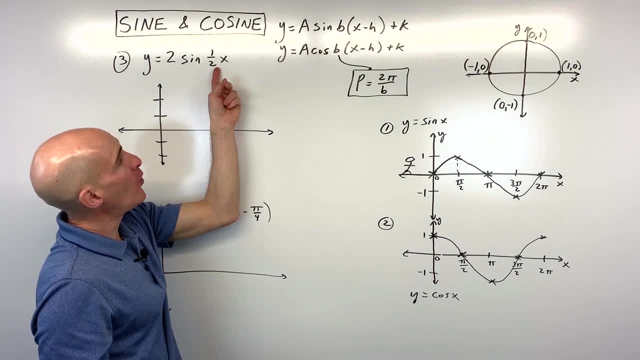 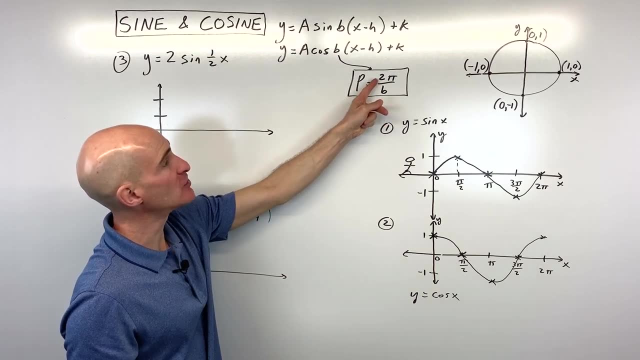 by 2.. But what does this 1 half do? Well, the 1 half is related to the period. through this formula: 2 pi divided by b. So you can see, if we were to put 1 half in here: 2 pi divided by 1 half. well, when you 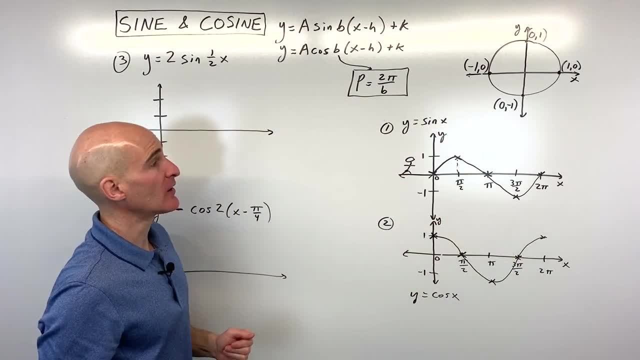 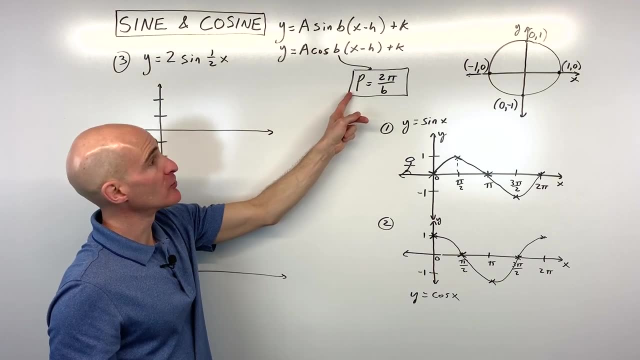 to happen is it's going to be a vertical stretch of the sine graph by 2.. Okay, you're multiplying all the y values by 2.. But what does this 1 half do? Well, the 1 half is related to the period through this formula: 2 pi divided by 2.. 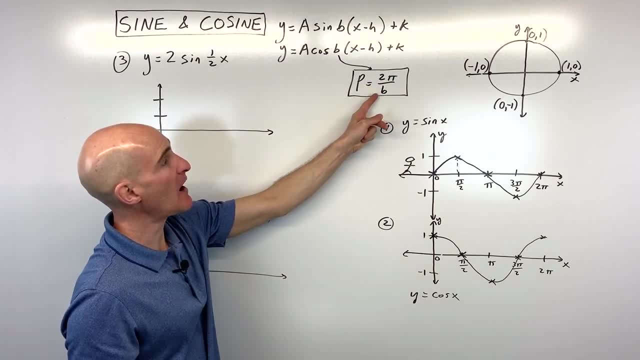 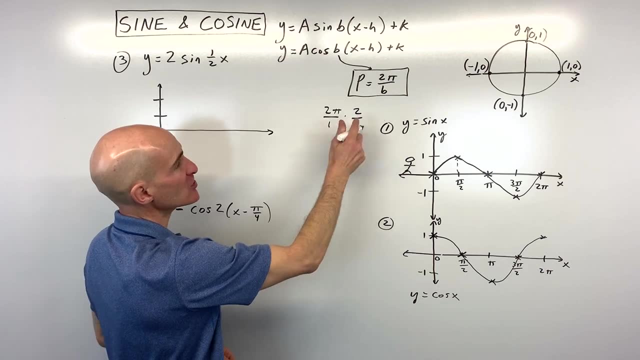 So you can see, if we were to put 1 half in here, 2 pi divided by 1 half- Well, when you divide it's like multiplying by the reciprocal. So it's really like multiplying by the reciprocal of 1 half, which is 2.. And you can see that's going to come out to a period of 4 pi. So 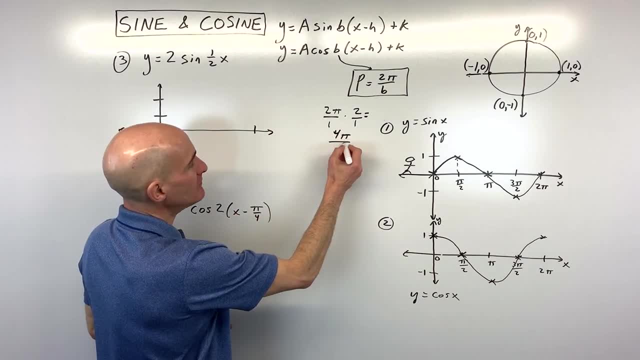 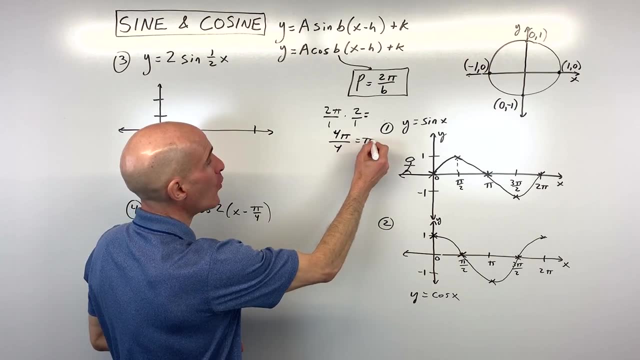 what I like to do next is I like to take that 4 pi, excuse me, and divide it by 4, because that's going to give us the scale on the horizontal axis. So 4 pi divided by 4 gives us 1 pi. 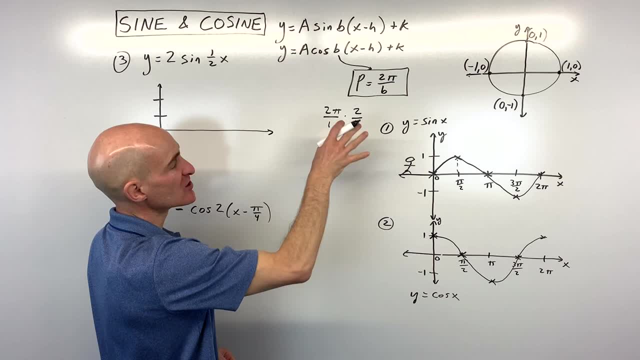 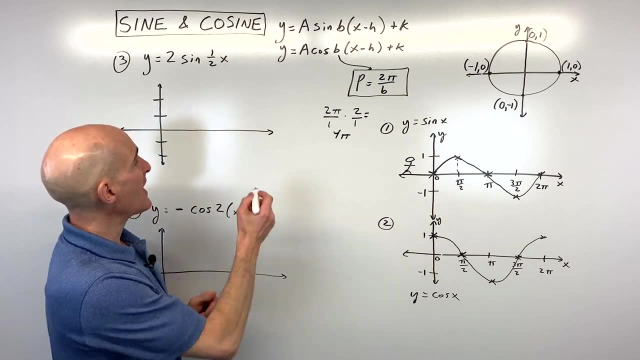 divide. it's like multiplying by the reciprocal. So it's really like multiplying by the reciprocal of 1 half, which is 2.. And you can see that's going to come out to a period of 4 pi. So what I like to do next is I like to take that 4 pi and divide it by 4, because that's going. 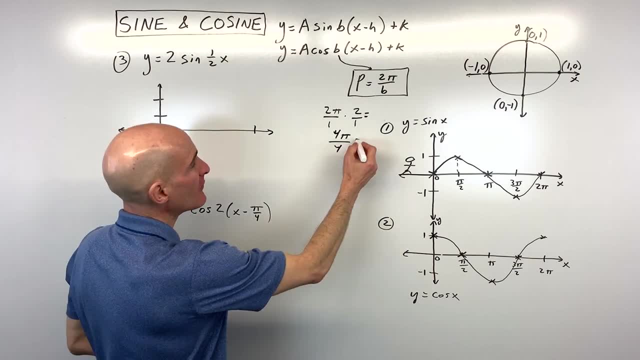 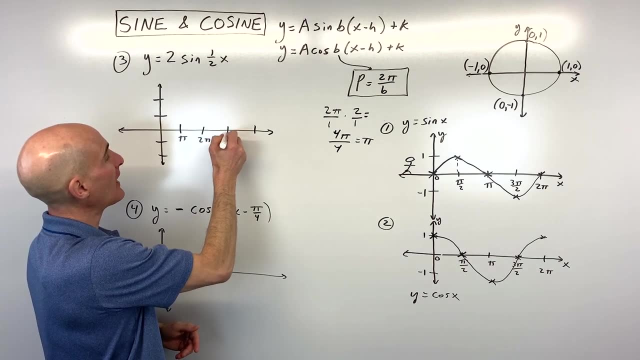 to give us the scale on the horizontal axis. So 4 pi divided by 4 gives us 1 pi. So what I'm going to do is I'm going to count per pi, 2 pi, 3 pi, 4 pi, just like you see over here, where we divide it up into quarters 1,, 2,. 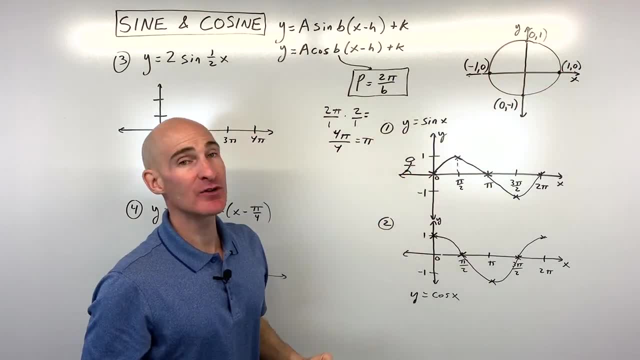 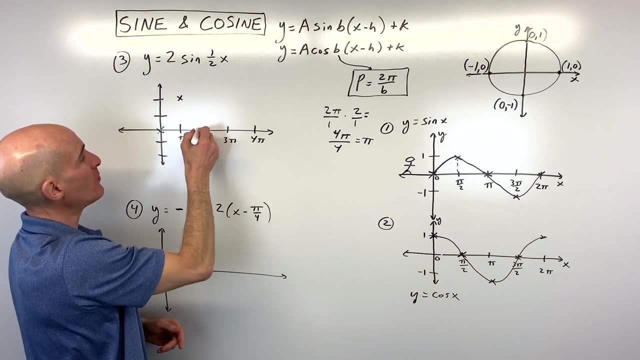 3,, 4,, just like the quadrants, see 1,, 2,. ok, dividing up into fourths. Again, we know that sine starts at the midline, so right here it goes up to the maximum, that's 2, back. 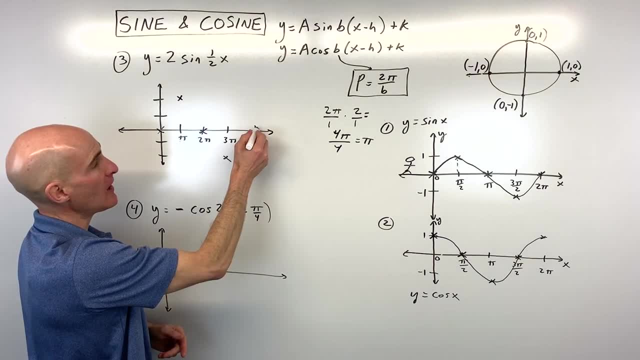 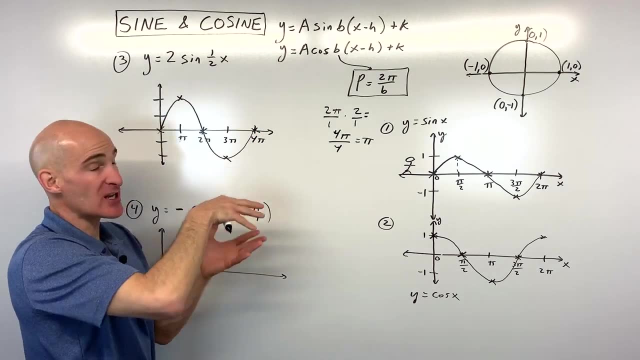 to the midline, down to the minimum that's here at negative 2, back to the midline and that's going to give us our basic, you know, shape of our sine graph. The only difference is it's been stretched by 2 in the vertical direction. it's also been stretched in the 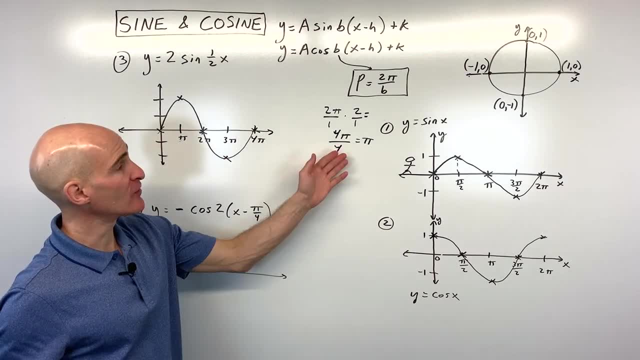 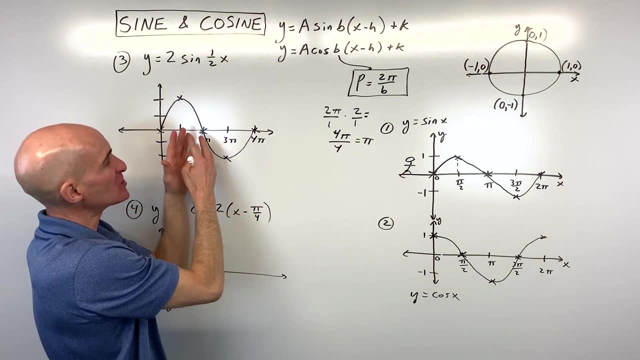 horizontal direction by 2, and again, we figured that out because the 1 half here group with the x has the opposite effect on the graph and actually, instead of looks like you're dividing by 2, it's actually multiplying the x values by 2,. but what a lot of students. 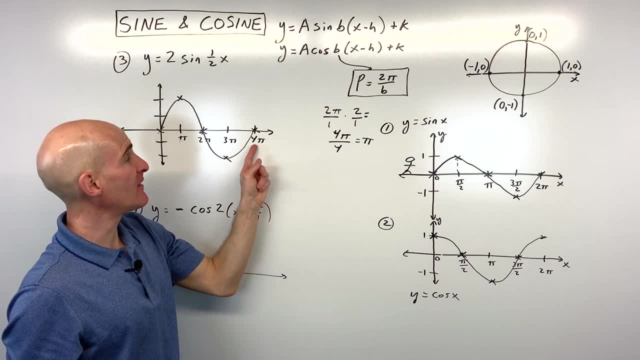 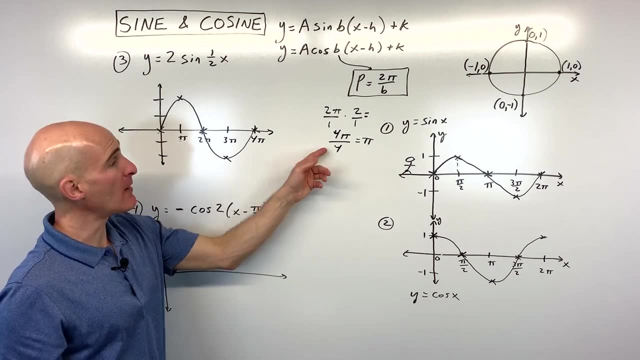 like to do is just use this formula, 2 pi over b to find the new period again. the period is how long it takes for it to complete one cycle before it repeats. then divide it by 4 or multiply by 1- fourth to get the new period. 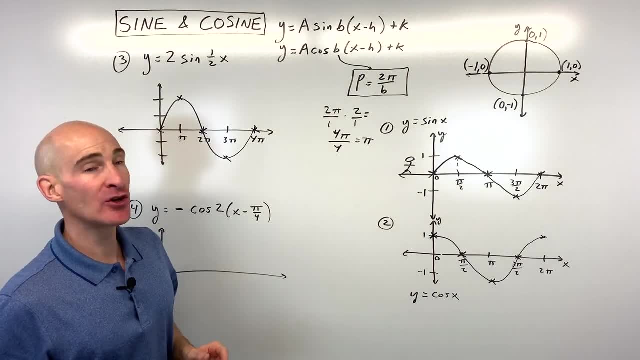 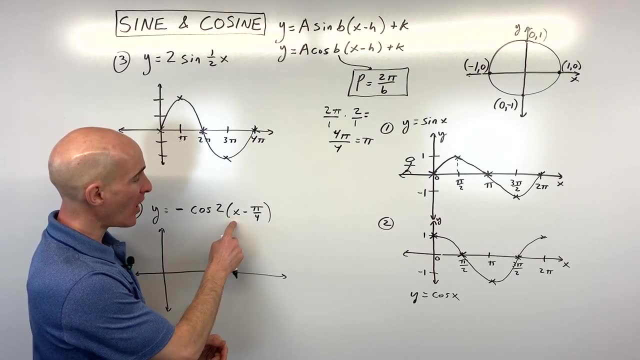 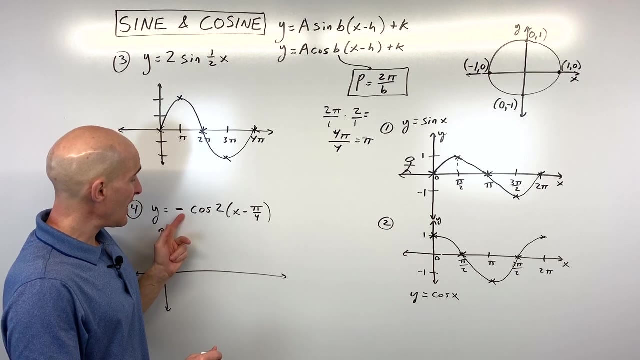 Okay, let's look at another example. see if you can do number 4. here we've got y equals negative cosine of 2 times the quantity x minus pi over 4.. Okay, a little bit more challenging here. what do you think the negative does to the graph? Well, the negative is going. 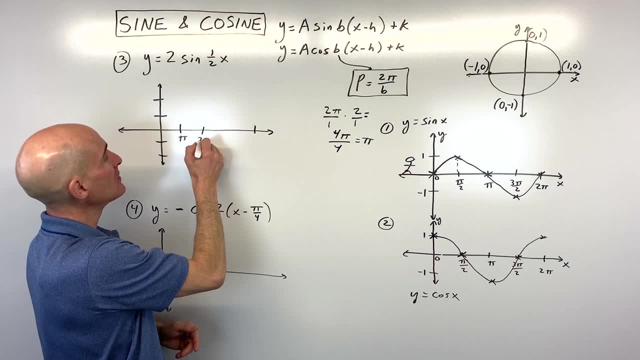 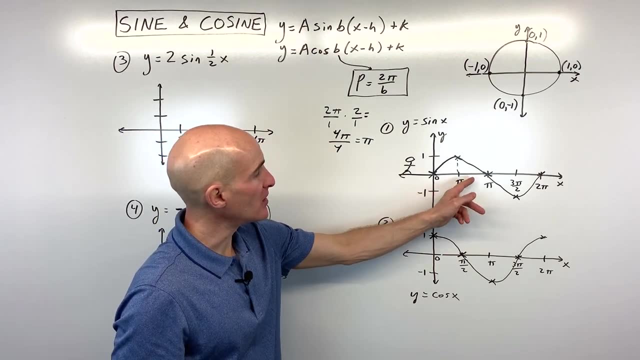 So what I'm going to do is I'm going to count by pi. So it's going to be 1 pi, 2 pi, 3 pi, 4 pi, just like you see over here, where we divided up into quarters 1, 2,, 3, 4, just like the quadrants, see 1, 2,. okay, dividing up into. 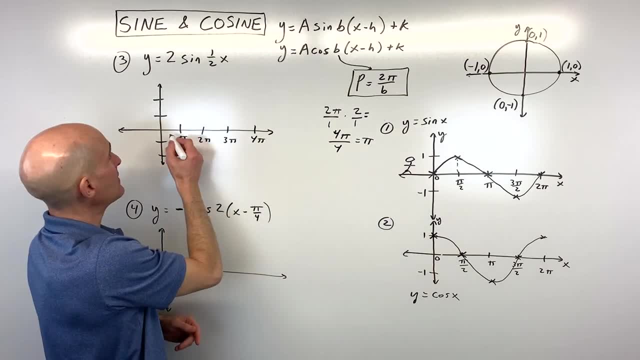 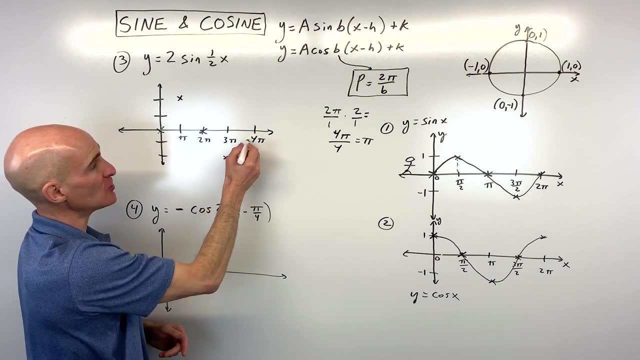 fourths, Again, we know that sine starts at the midline. so right here it goes up to the maximum, that's 2, back to the midline, down to the minimum, that's here at negative 2, back to the midline, and that's going to give us our basic, you know, shape of our 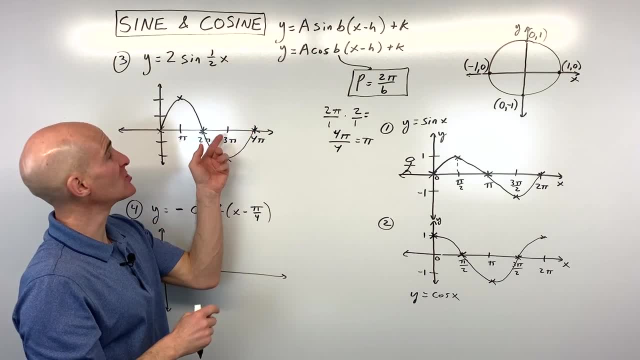 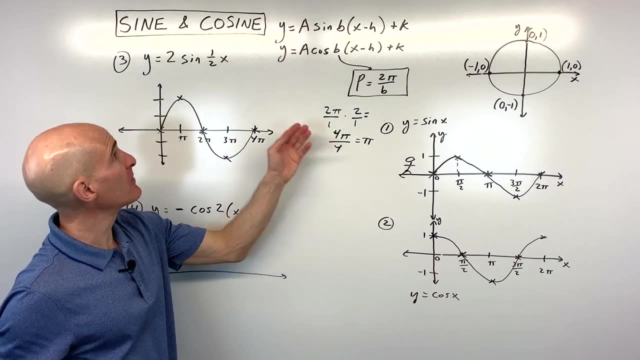 sine graph. So we've stretched by 2 in the vertical direction. It's also been stretched in the horizontal direction by 2.. And again, we figured that out because the one-half here group with the x has the opposite effect on the graph. It actually, instead of it, looks like you're. 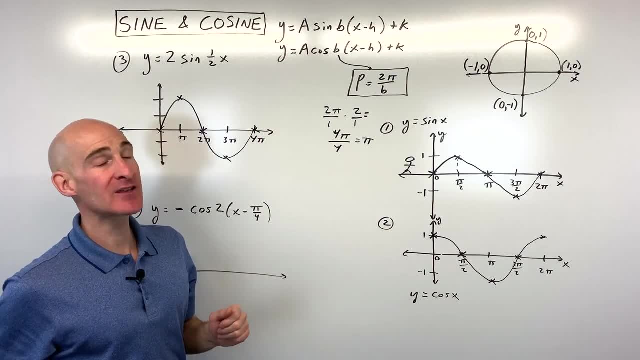 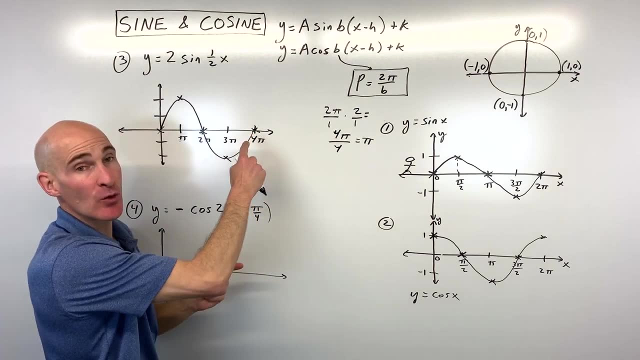 dividing by 2, it's actually multiplying the x values by 2.. But what a lot of students like to do is just use this formula, 2, pi over b- to find the new period. Again, the period is how long it takes for it to complete one cycle before it repeats, Then divide it. 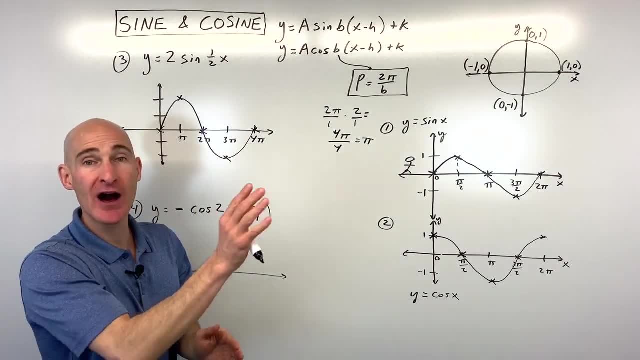 by 4, or multiply it by one-fourth to get the scale, like what you're doing here. So you 're counting by each of those quarters. Okay, let's look at another example. See if you can do number 4 here We've got y equals. 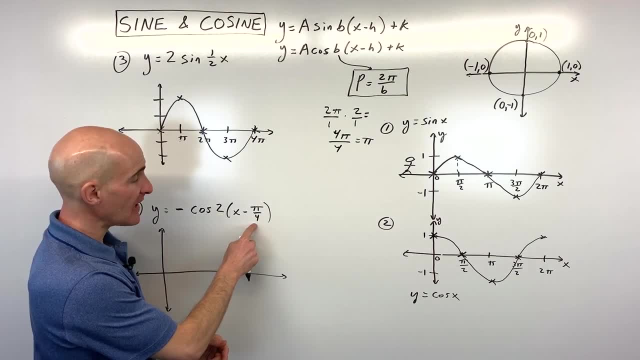 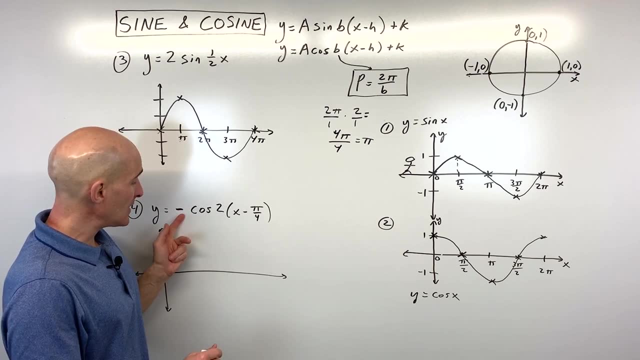 negative cosine of 2 times the quantity x minus pi over 4.. Okay, a little bit more challenging here. What do you think the negative does to the graph? Well, the negative is going to make all the y values the opposite sign, so it's going to actually reflect it over. 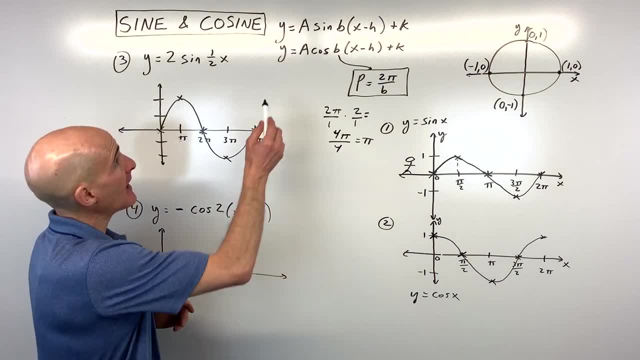 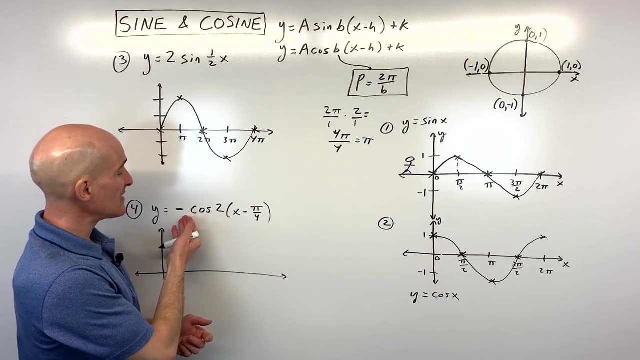 the x-axis. okay, Now when you talk about the amplitude- this number here that comes in front of the sine or the cosine- the amplitude is always positive. So if your teacher says what's the amplitude Here, you would say the amplitude's 1. Here. 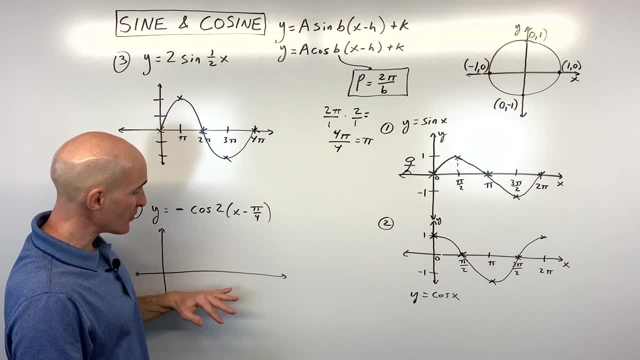 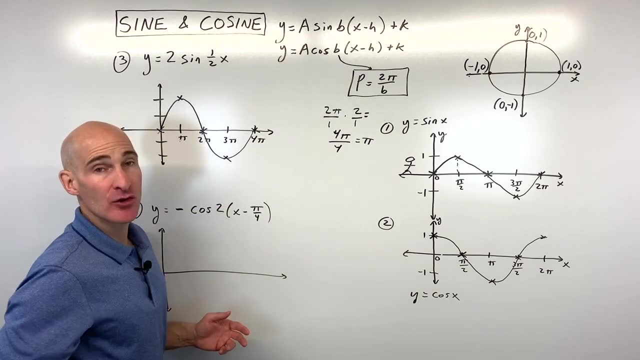 to make all the y values the opposite sine, so it's going to actually reflect it over the x axis. okay, Now, when you talk about the amplitude, this number here that comes in front of the sine or the cosine, the amplitude is always going to be the same. it's going. 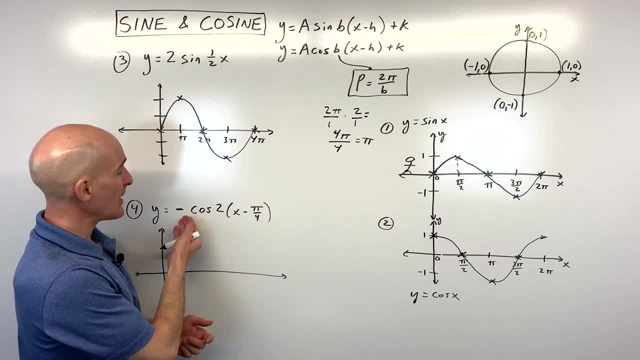 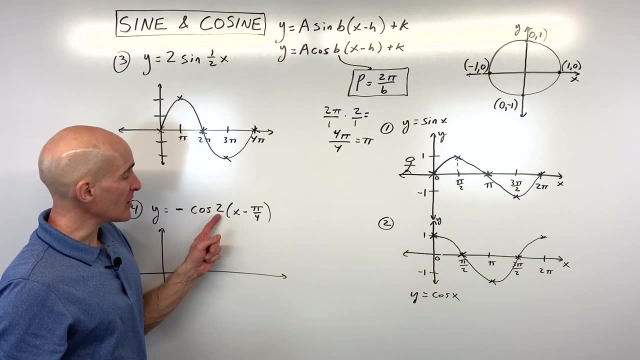 to be positive. So if your teacher says what's the amplitude? here you would say the amplitude is 1, here you'd say the amplitude is 2, it's always positive. this negative is just reflecting it. Okay, now let's go to the period. so we're going to use this formula again: 2 pi divided. 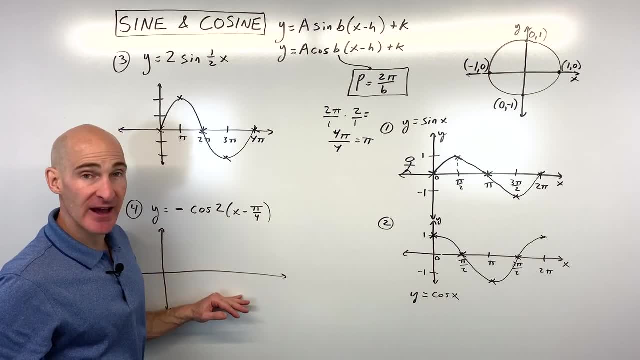 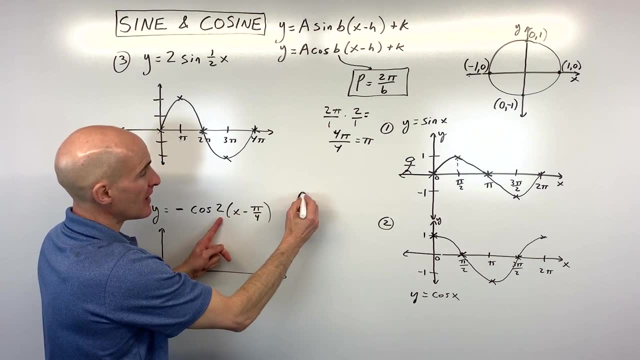 you'd say the amplitude's 2.. It's always positive. This negative is just reflecting it. Okay, Now let's go to the period. So we're going to use this formula again: 2 pi divided by b, b is 2, so that means that period is going to be 2 pi divided by 2, which is pi. okay. 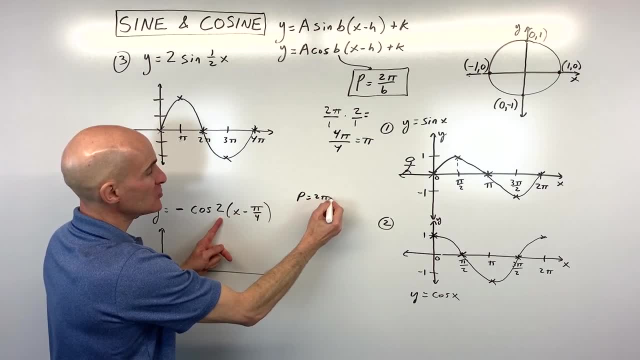 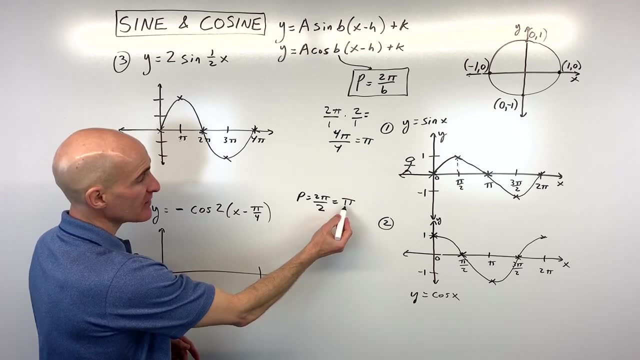 by b. b is 2,, so that means that the period is going to be 2 pi divided by 2, which is pi okay. and so then, what I'm going to do is I'm going to figure out the scale by multiplying. 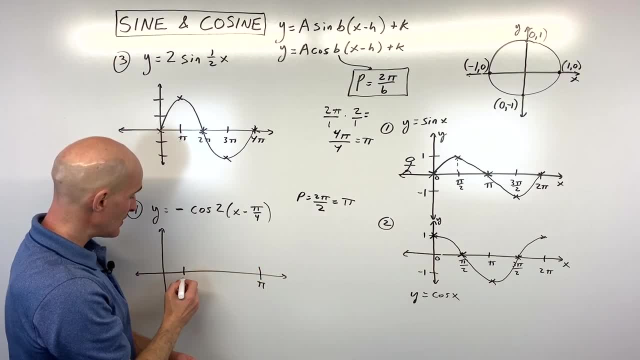 this by 1, fourth, or dividing by 4.. So that's going to be pi divided by 4, 2 pi divided by 4, which is pi over 2,, 3 pi over 4, and then 4 pi over 4,, which is pi. so we're always 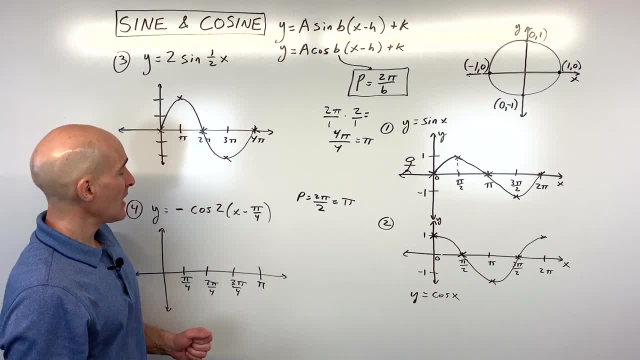 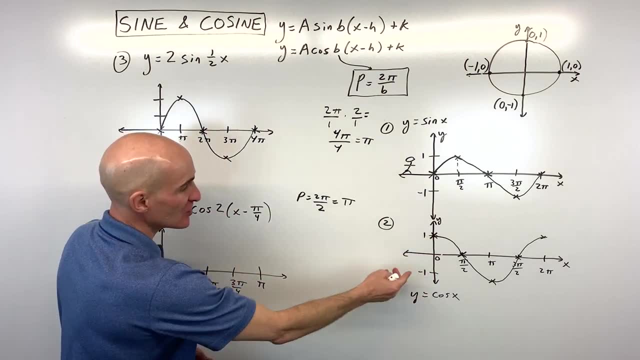 dividing up into fourths. But now we're working with cosine and when we think about cosine, we know that cosine normally starts at the maximum value, right. But because it's being reflected because of this negative, it's going to start down here at the minimum value, right. 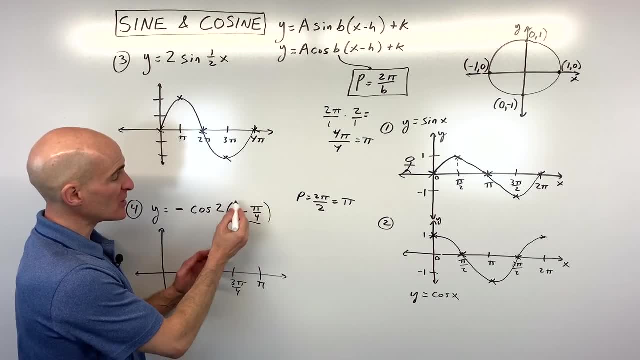 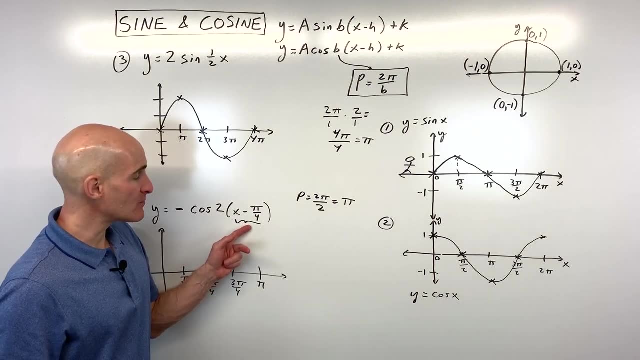 But what about this pi over 4?? Well, the pi over 4, okay, when it's grouped with the x like this, it's shifting it in the horizontal direction left and right, but this actually affects So the minus pi over 4 is actually going to pick up the graph and shift it to. 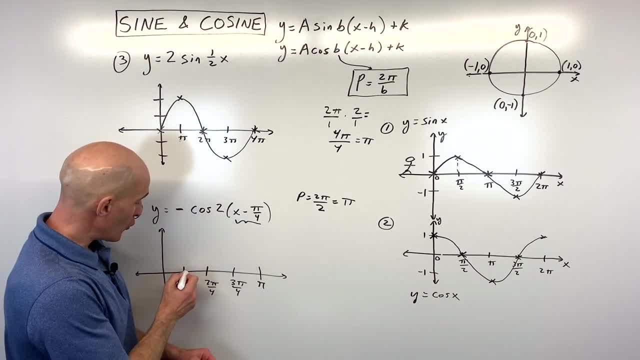 the right pi over 4.. What I like to do is I like to draw like an open circle. okay, and I'm going to think of this as my new origin. So if I wanted to, I could kind of draw in like a dotted line. This is kind of like my new y-axis, this is kind of like you know. 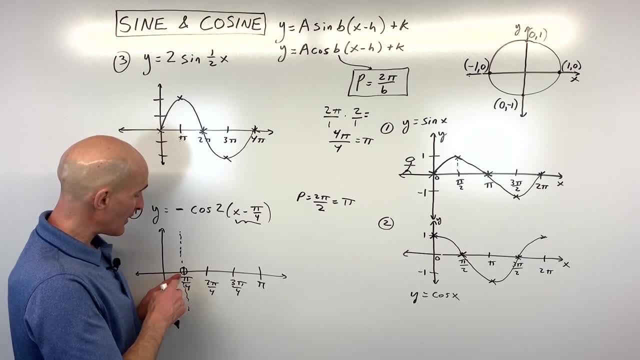 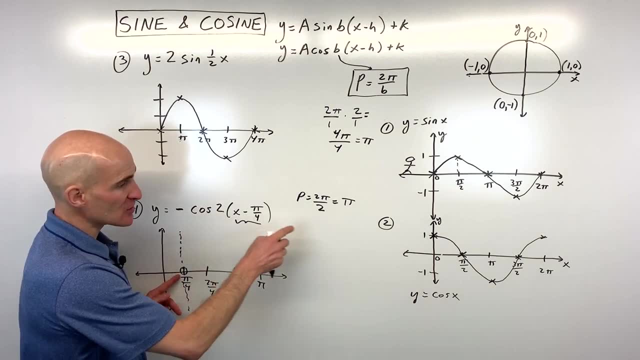 my x-axis, and this is like my origin or my starting point. So, now that I've taken the shift into account, all I have to do now is graph, my basic cosine graph. but keep in mind that it's reflected, so it's going to start down here, So it's going to start over here. 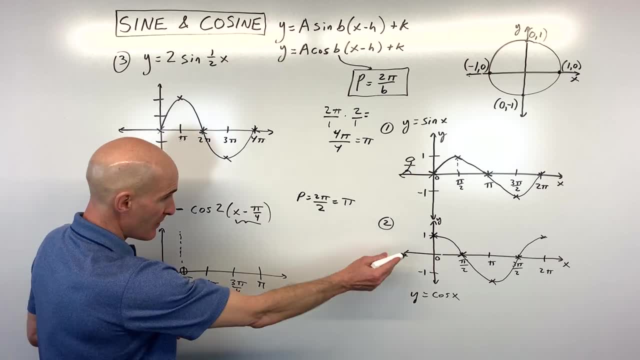 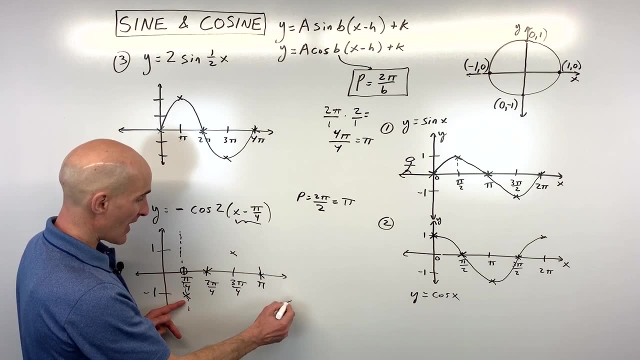 at negative 1, then it's going to go back to the midline, up to the maximum positive 1, back to the midline and then over here back to the minimum. This is going to be at 5 pi over 4, and now, if we draw our graph, we've got it. Now you can draw more points. 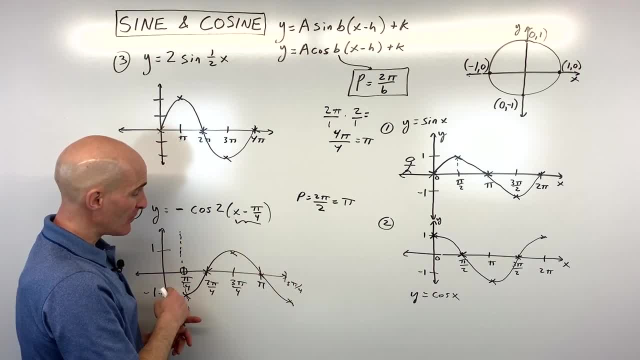 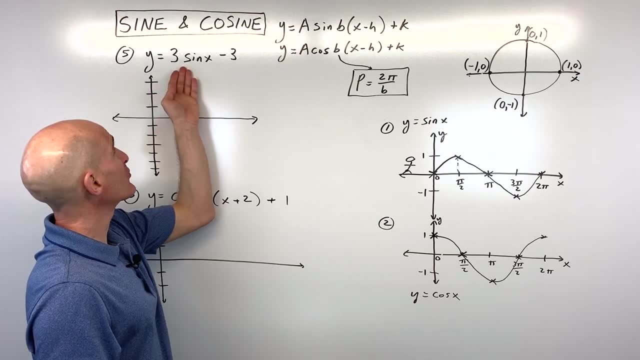 and continue on that graph in both directions. but this is one period or one cycle. Let's do a couple more examples. Okay, see if you can do number 5.. We've got y equals 3 sine x minus 3.. How would you graph that one? Well, the first thing I want you to notice, 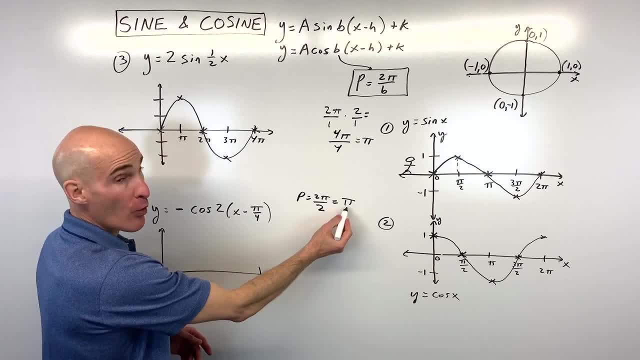 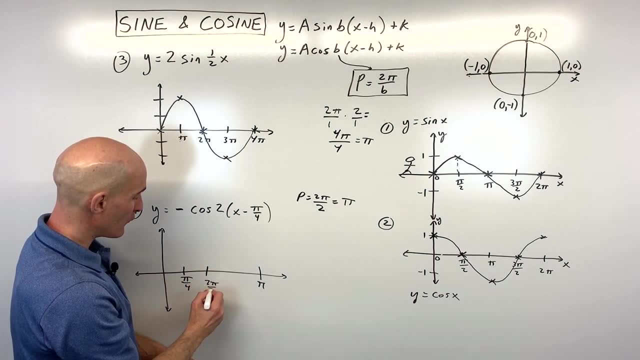 And so then, what I'm going to do is I'm going to figure out the scale by multiplying this by one-fourth, or dividing by 4.. So that's going to be pi divided by 4, 2 pi divided by 4, which is pi over 2, 3 pi over 4, and then 4 pi over 4, which is pi. So we're always 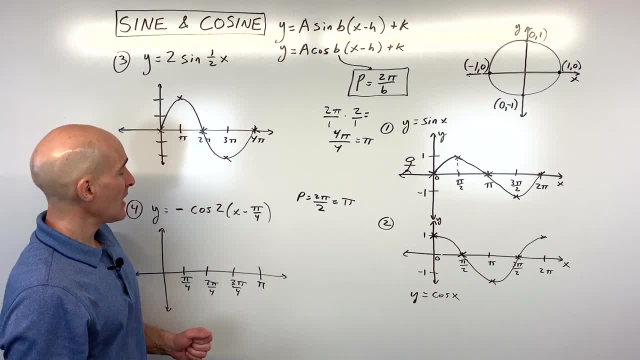 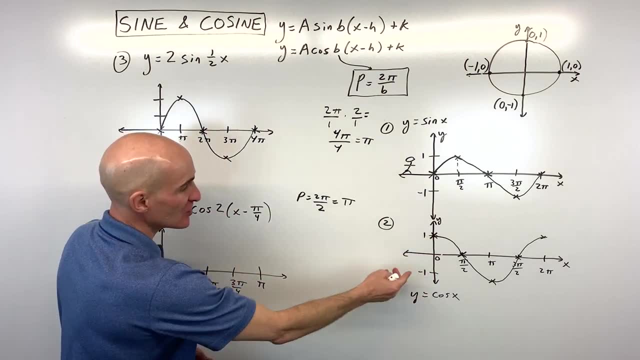 dividing up into fourths. But now we're working with cosine and when we think about cosine, we know that cosine normally starts at the maximum value, right. But because it's being reflected because of this negative, it's going to start down here at the minimum value, right. 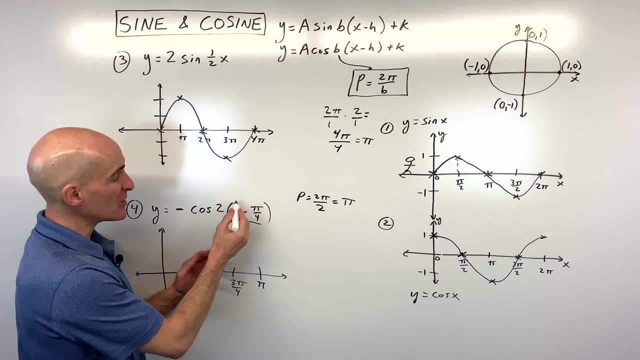 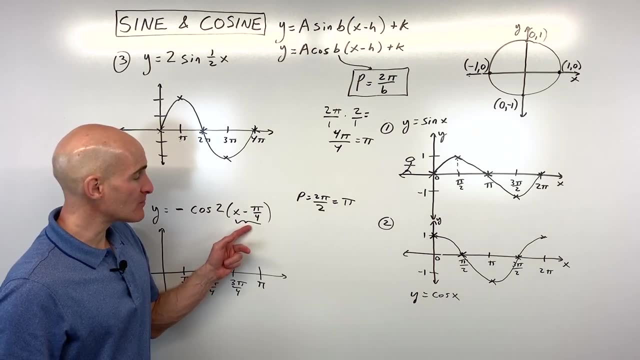 But what about this pi over 4?? Well, the pi over 4, okay, when it's grouped with the x like this. it's shifting it in the horizontal direction left and right. But this actually has the opposite effect. This pi over 4 is actually going to pick up the graph and shift it to the right pi over. 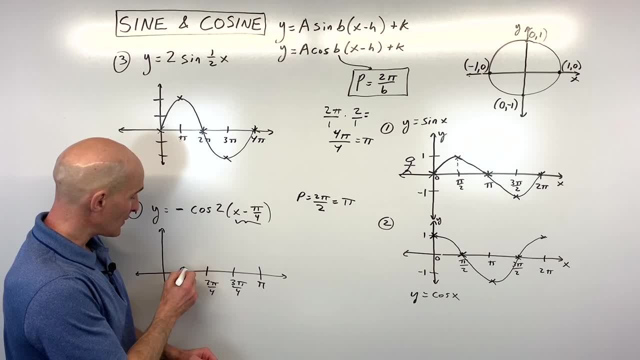 4. What I like to do is I like to draw like an open circle. okay, And I'm going to think of this as my new origin, So if I wanted to, I could kind of draw in like a dotted line. This is kind of like my new y-axis, This is kind of like, you know, my x-axis And this. 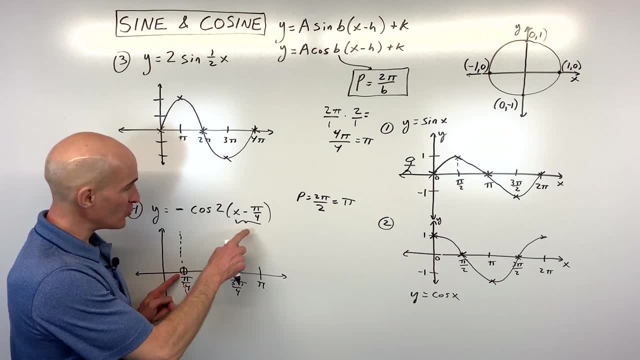 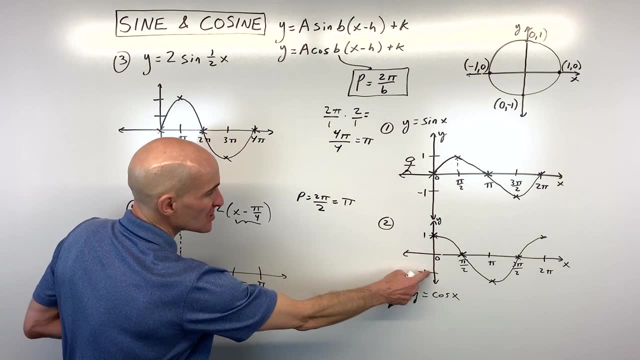 is like my origin or my starting point. So, now that I've taken the shift into account, all I have to do now is graph, my basic cosine graph. but keep in mind that it's reflected, so it's going to start down here, So it's going to start over here at negative 1, and 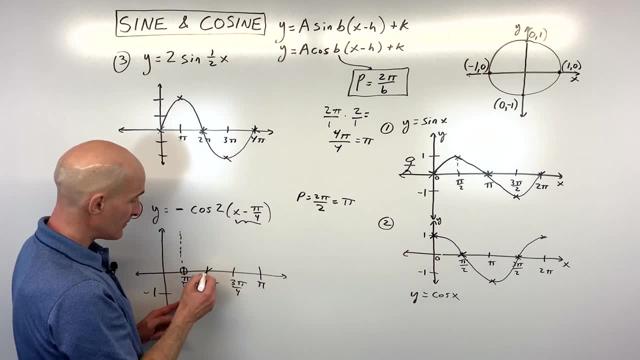 then it's going to go back to the midline, up to the maximum positive 1, back to the midline and then over here back to the minimum. This is going to be at 5 pi over 4.. And now, 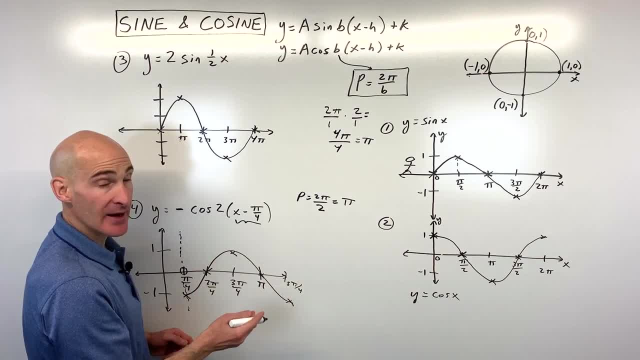 if we draw our graph, we've got it. Now you can draw more points and continue on that graph in both directions, but this is one period or one cycle. Let's do a couple more examples. Okay, see if you can do number 5.. We've got: y equals 3 sine pi over 4.. Okay, so this is. going to be at 5 pi over 4.. Okay, see if you can do number 5.. We've got y equals 3 sine pi over 4.. Okay, see if you can do number 5.. We've got y equals 3 sine pi over 4.. Okay, see. if you can do number 5.. We've got y equals 3 sine겠지만 pi over 4.. Okay, see if you can do number 5.. We've got y equals 3 sinepi over 4.. Okay, see if you can do number 5.. 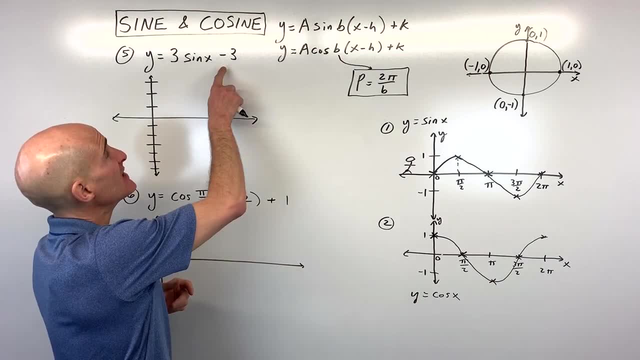 Okay, see if you can do number 5.. Okayus, 3 mustard然後 pi over 4 over 3.. Now think about something. Let's put a allá公ور. Now think about something. See, let's talk about something again, because this is slime class. Let's do our difficult. math here A day again. now let's just get this through out. So we're going to bring in 3 pi over 4, and then 5 pi over 4, so 3 studios out. Okay, so divided by 5 pi over. 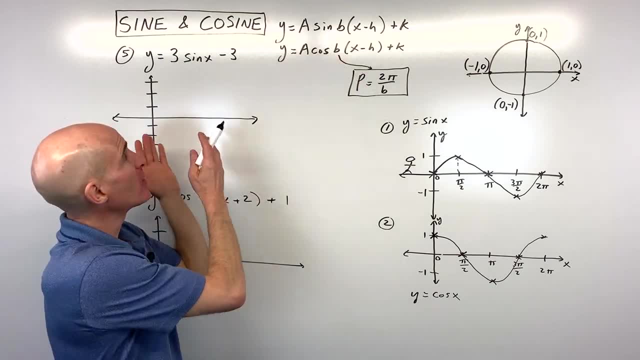 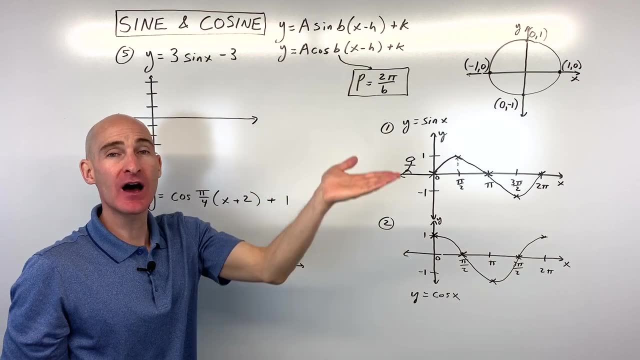 4,. okay, See if I can do number 5, let's go through this a little bit. and we've got parentheses, like you see here. then it would be what we call a phase shift, left and right. okay, but because the three is not grouped with the x, this tells us that it's a vertical shift up and 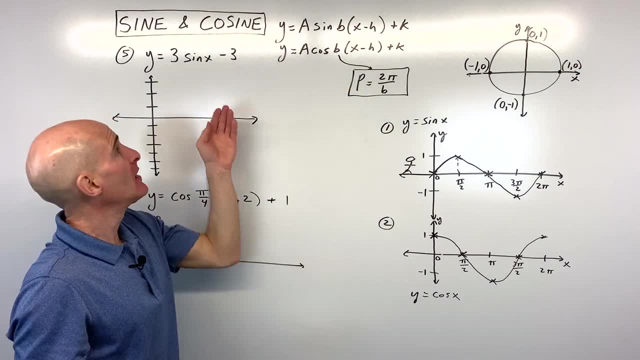 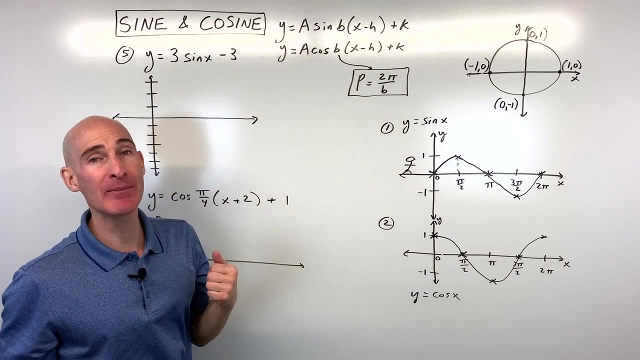 down. the minus three is going to shift it down three. if it was plus three would shift it up three. this k value has the same effect as the sign, whereas the one group with the x- remember that- has the opposite effect. so here, what i like to do- because it's minus three, shifted down three- is i: 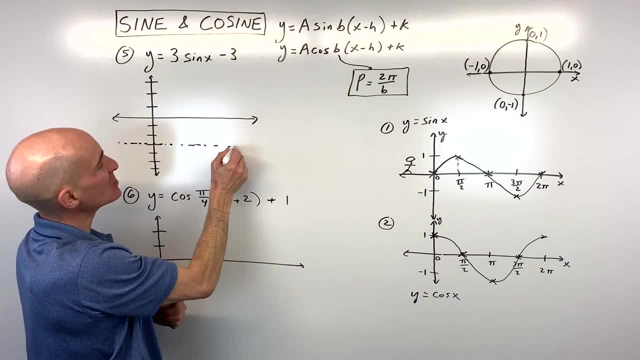 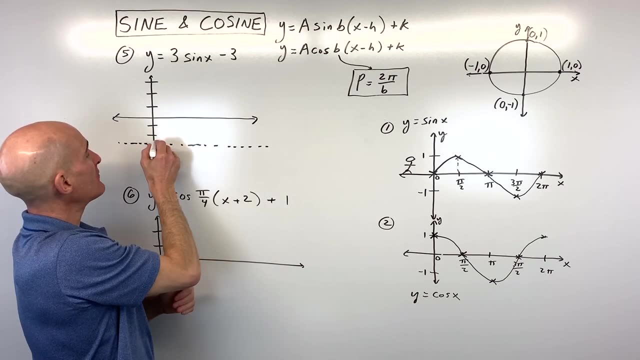 like to go down three and i like to draw like a dashed or dotted line. i'm going to think of this as our new x-axis- okay, it's not shifting left or right, so i'm going to think of this point, right here, at negative three, as our new origin or our new starting point. now all i have to do is focus. 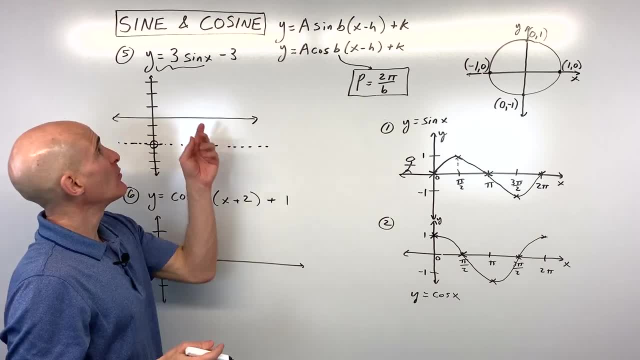 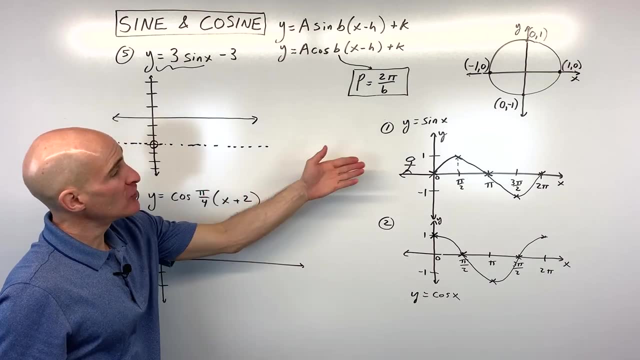 on what's left, which is y equals three sine of x, and we know the three already- is the amplitude, that's the vertical stretch. it's stretching it by three in the y direction, and all we have to do now, if we are familiar with our sine graph. 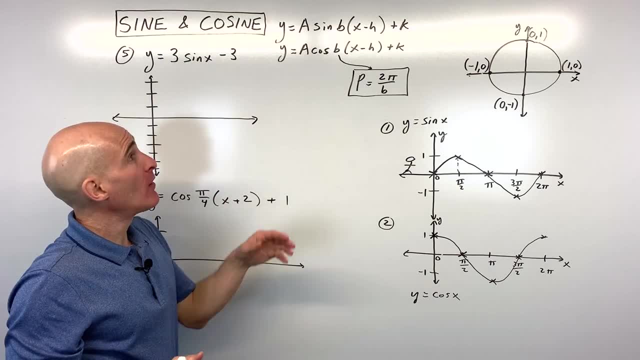 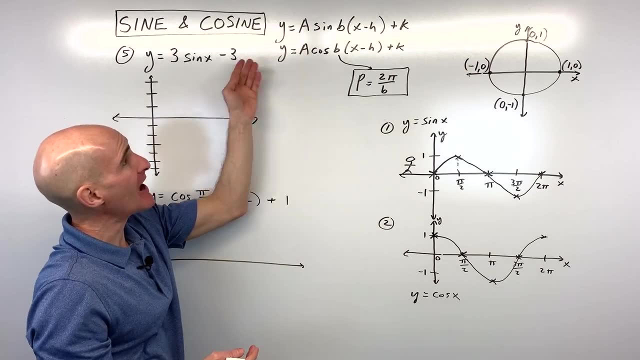 is? is this 3 grouped with this x? Well, if it was in parentheses, like you see here, then it would be what we call a phase shift, left and right. Okay, but because the 3 is not grouped with the x, this tells us that it's a vertical shift up and down The minus 3. 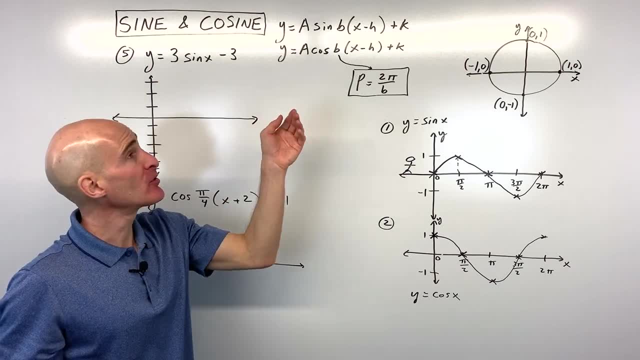 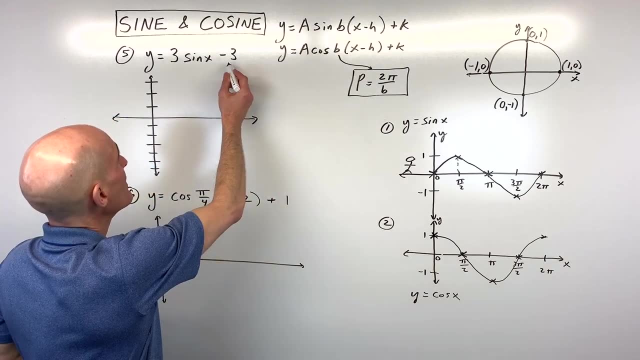 is going to shift it down 3.. If it was plus 3, it would shift it up 3.. This k value has the same effect as the sine, whereas the one grouped with the x- remember that- has to be the opposite effect. So here what I like to do: because it's minus 3, shifted down 3,. 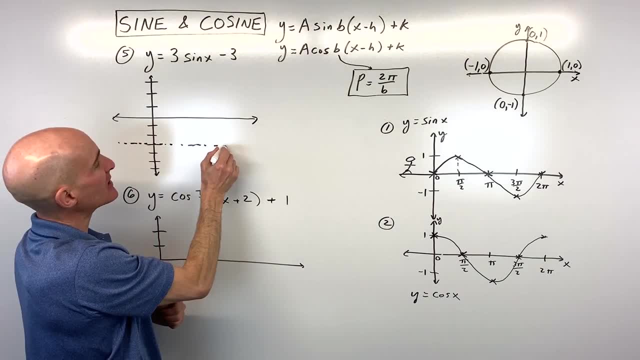 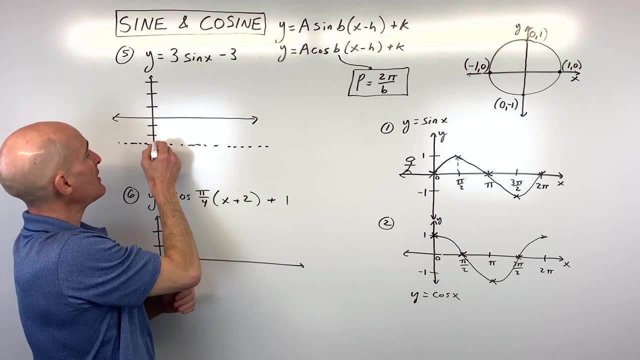 is. I like to go down 3, and I like to draw a dashed or dotted line. I'm going to think of this as our new x axis. Okay, it's not shifting left or right, so I'm going to think of this point, right here, at negative 3, as our new origin, our new starting point Now. 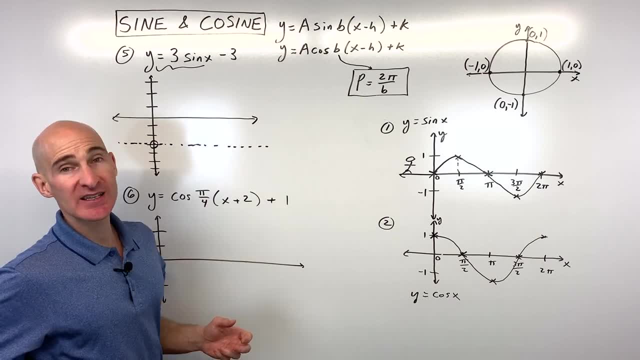 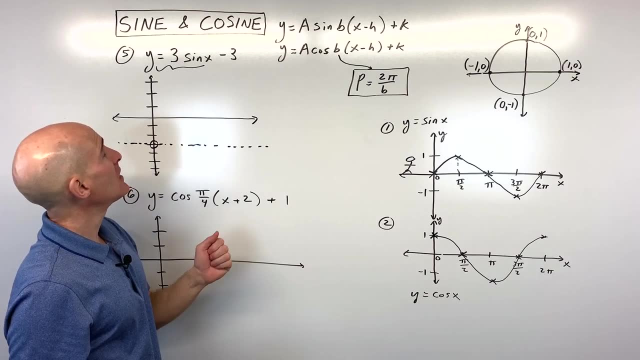 all I have to do is focus on what's left, which is y equals 3 sine of x, and we know the 3 already is the amplitude, that's the vertical stretch, it's stretching it by 3.. And the y direction. And all we have to do now, if we are familiar with our sine graph. 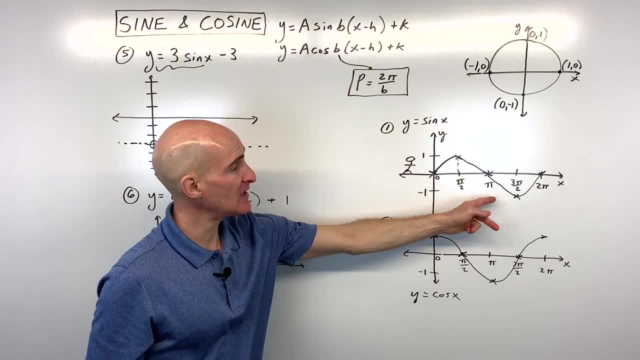 is graph, the sine graph, and instead of going up to 1, we're going to go up to 3.. Instead of going down to negative 1, we're going to go down to negative 3.. Okay, so, let's go ahead. 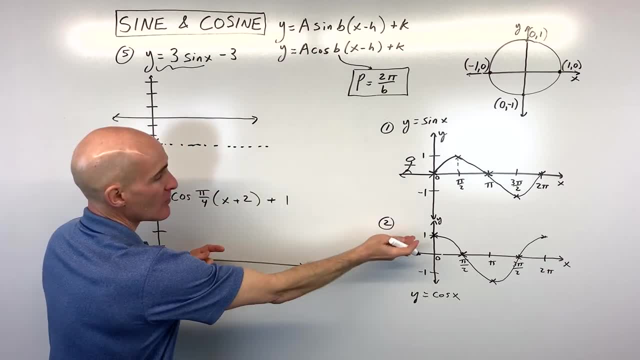 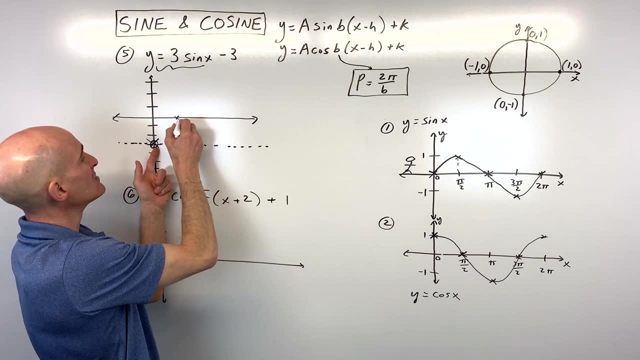 and do that. So it starts at the midline. okay, for sine Cosine, remember starts at the maximum. Then we're going to go up to the maximum, okay, which is going to be here at 0.. Okay, I went up 3.. Then we're back to the midline, Then we're down to the minimum. 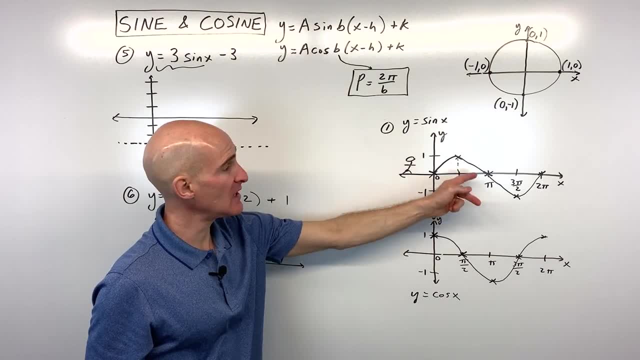 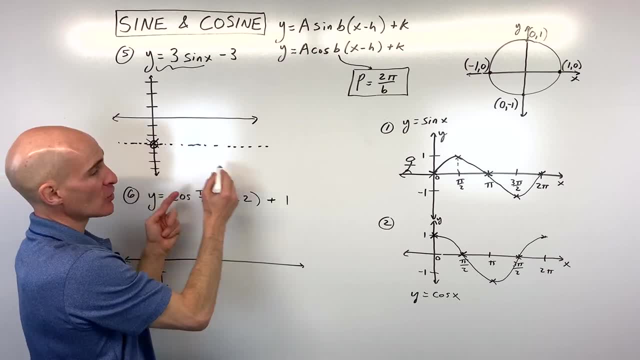 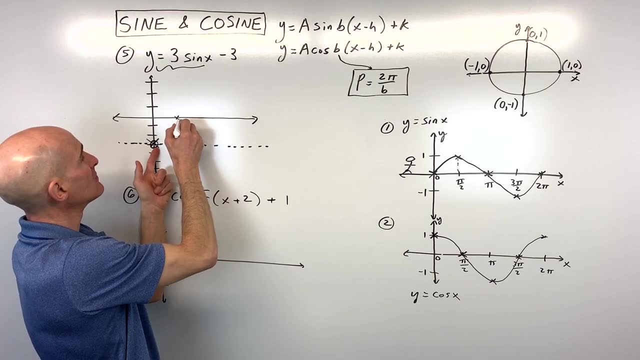 let's go ahead and do that. so it starts at the midline, okay, for sine cosine, remember, starts at the maximum. then we're going to go up to the maximum, okay, which is going to be here at zero. okay, i went up three, then we're back to the midline, then we're down to the minimum, which is. 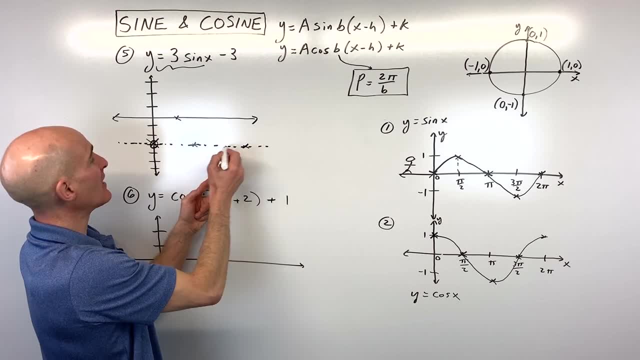 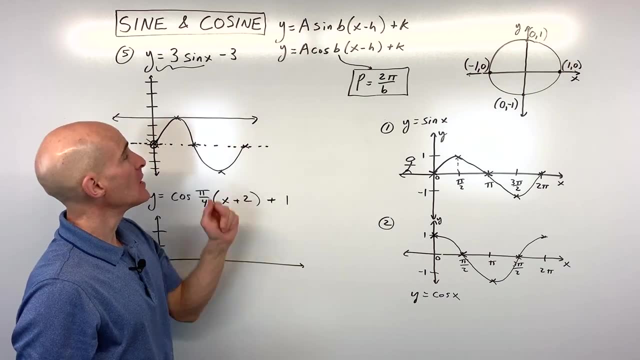 going to be three below that midline, and then we're back to the midline. okay, now, the only thing that i didn't put in this uh yet are the, the scale, the x values here. so what we want to do is we want to look at the number that comes in. 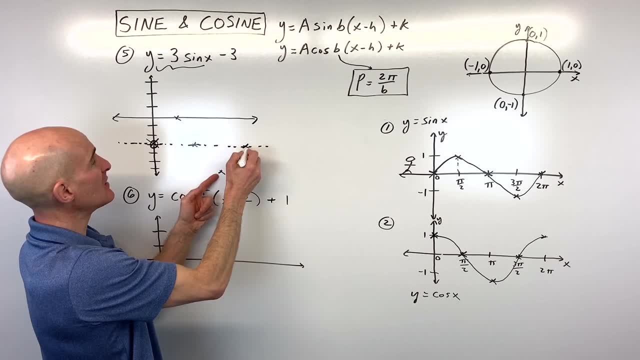 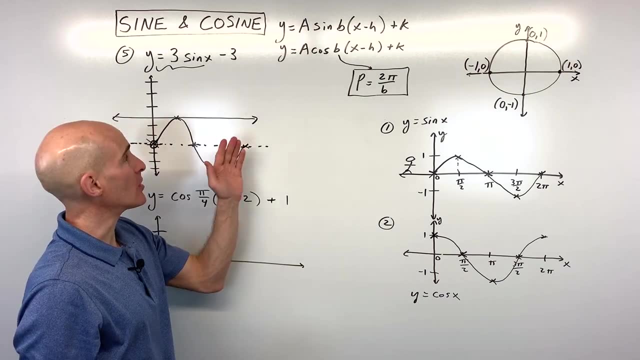 which is going to be 3 below that midline, And then we're back to the midline. Okay, now, the only thing that I didn't put in yet are the scale, the x values here. So what we want to do is we want to look at the number. 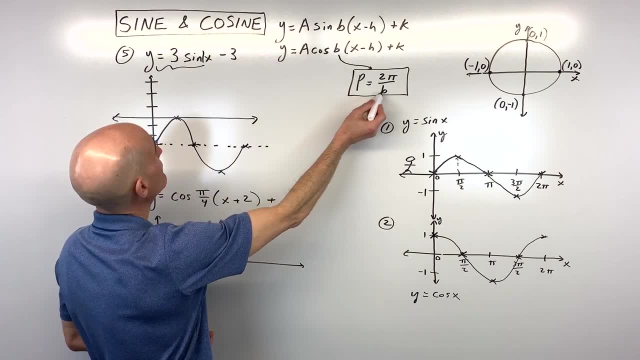 that comes in front of x, that's 1.. We want to use the formula 2 pi divided by b. that b is 1.. So 2 pi divided by 1 is 2 pi. Okay, so that's going to be our period, And then. 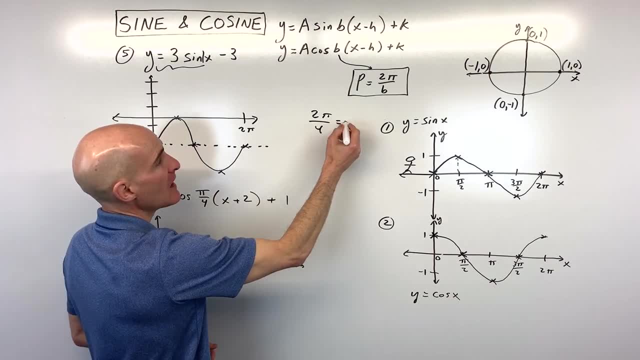 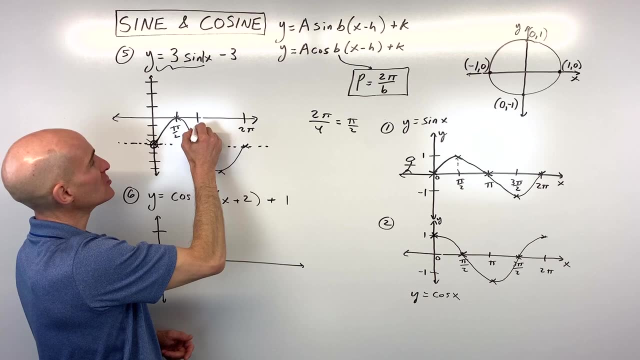 we want to divide that by 4, or multiply by 1, fourth, and that's going to give us a scale of pi over 2, once we reduce. So we're counting here by pi over 2.. 2 pi over 2, which is pi. 3 pi over 2.. 4 pi over 2, which is 2 pi, and that gives us our 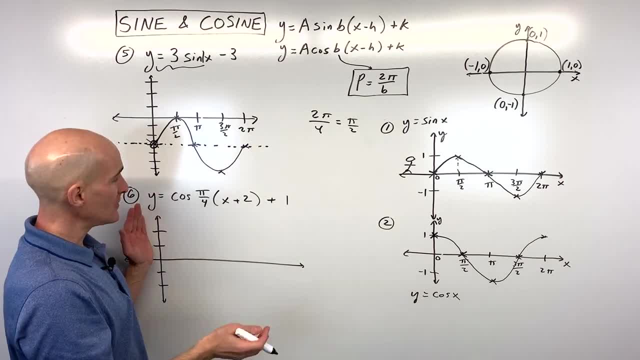 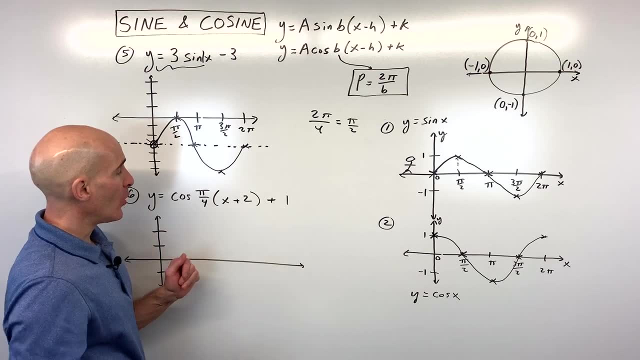 scale. Okay, let's go to number 6 now See if you can do this one. y equals cosine pi over 4 times the quantity x plus 2 plus 1.. Okay, so what do you think on this one? Well, 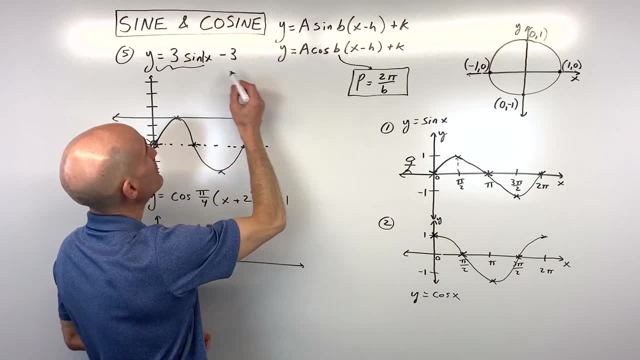 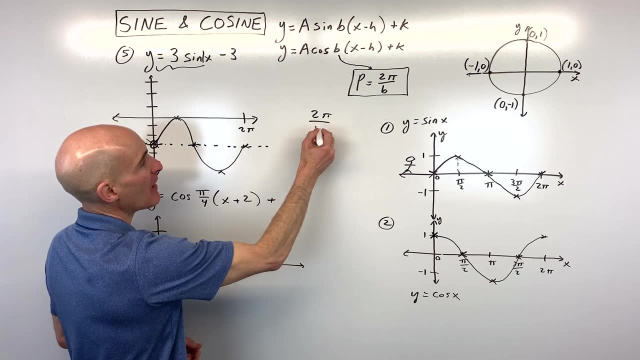 front of x, that's one. we want to use the formula two pi divided by b, that b is one. so two pi divided by one is two pi. okay, so that's going to be our period. and then we want to divide that by four, or multiply by one, fourth, and that's going to give us a scale of pi over two once we reduce. so we're. 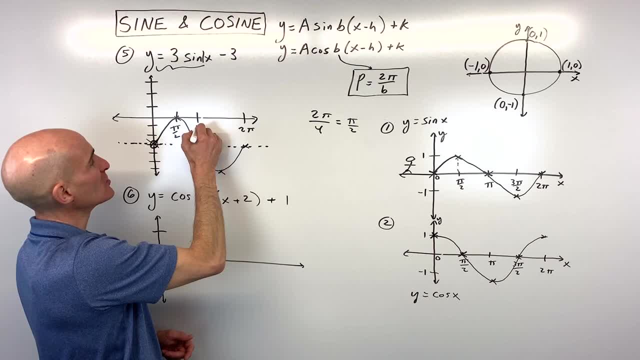 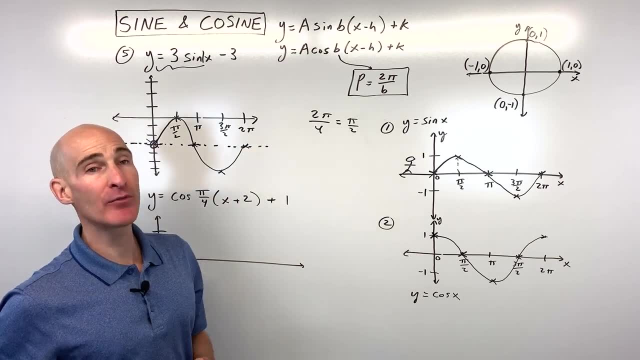 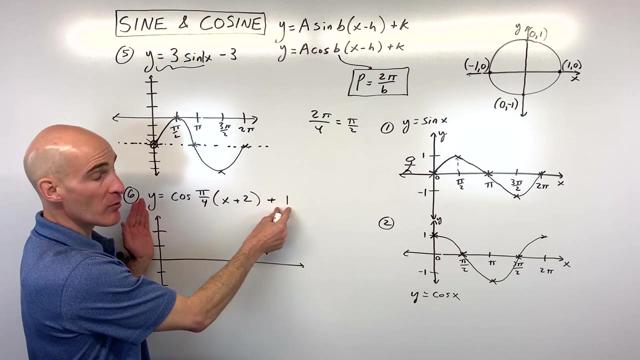 counting here by pi over two, two pi over two, which is pi three. pi over two, four pi over two, which is two pi, and that gives us our scale. okay, let's go to number six now see if you can do this. one y equals cosine pi over four times the quantity x plus two plus one. okay, so what do you think on this one? well, 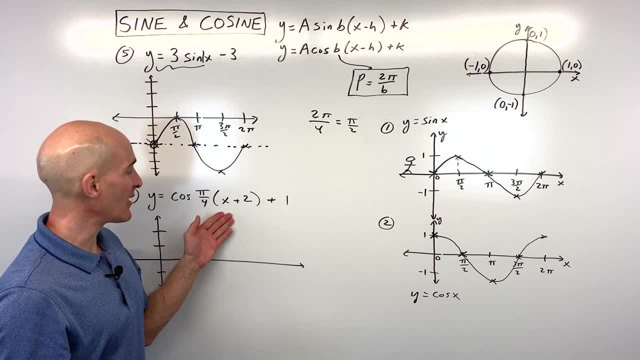 the first thing i like to do- and i didn't do it on this one, but what i like to do first- is i like to figure out what the period is so i can figure out what the scale is on our x-axis. so let's do that. 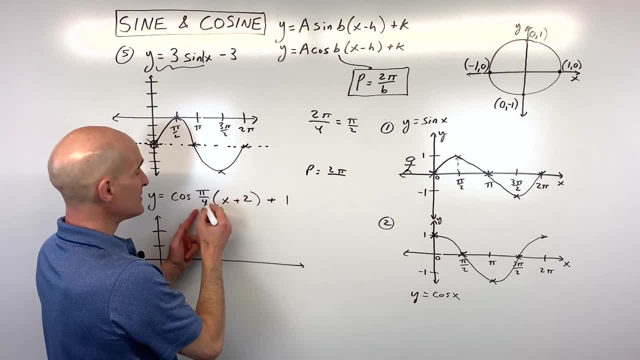 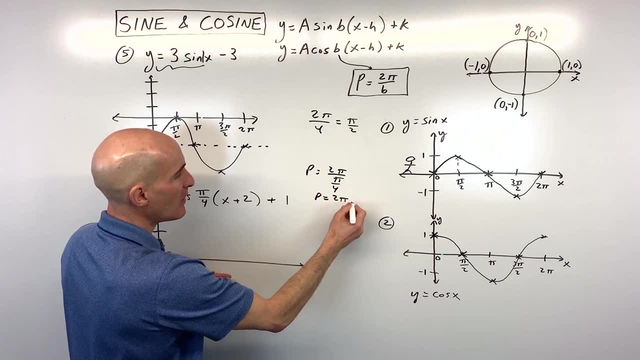 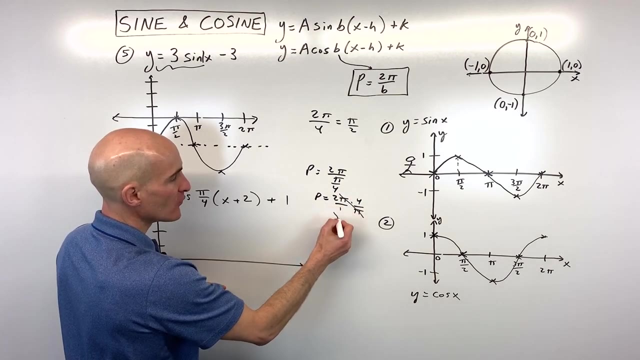 first, we've got: period equals two pi divided by pi over four. right, that's our b value. when we divide this by a fraction, it's like multiplying by the reciprocal. so this is really like two pi times four over pi. two pi is like two pi over one. see how the pi's cancel and two times four gives. 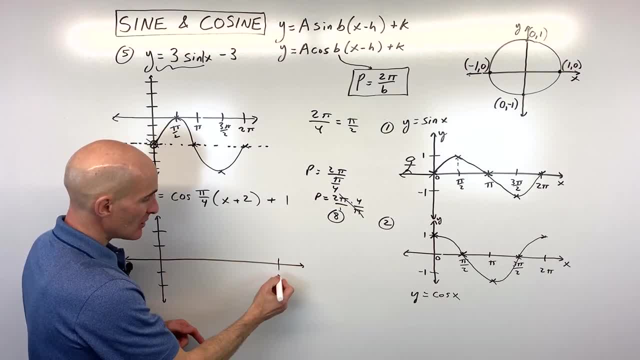 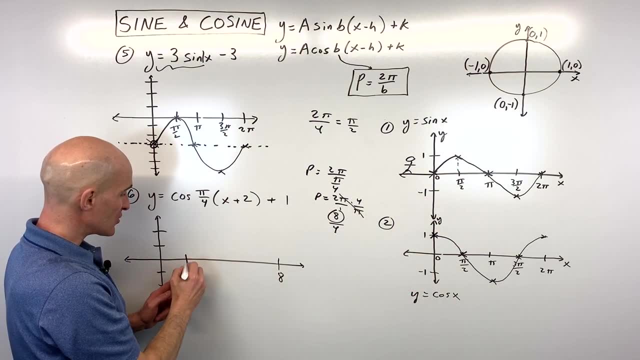 us a period of eight. so let's go to our x-axis here. let's call this eight. if we divide this by four- because, remember, we're dividing up into four pieces- this is going to give us a scale of two. so it's going to go two, four, six, eight. okay, so i just keep adding two each time. now what i like to do is: 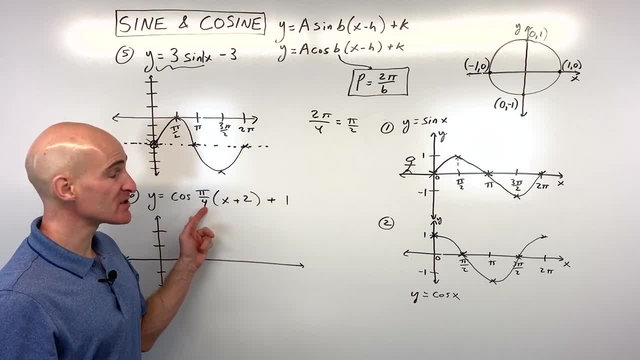 the first thing I like to do- and I didn't do it on this one, but what I like to do first- is I like to figure out what the period is So I can figure out what the scale is on our x-axis. So let's do that first. We've got period equals 2 pi over 2.. 2 pi over 2 is 2.. 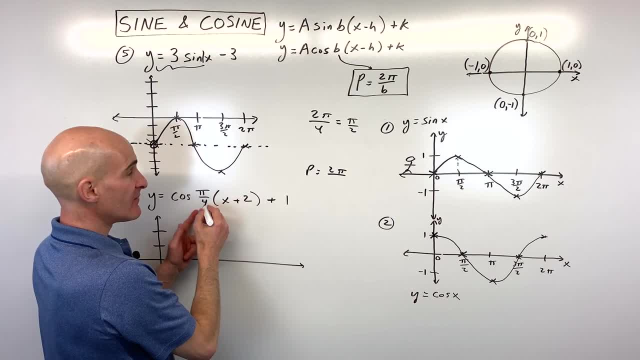 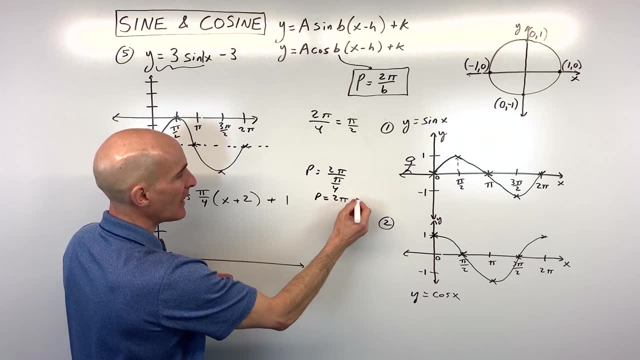 we've got period equals 2 pi divided by pi over 4, right, That's our b value. When we divide by a fraction, it's like multiplying by the reciprocal. So this is really like 2 pi times 4 over pi, 2 pi. 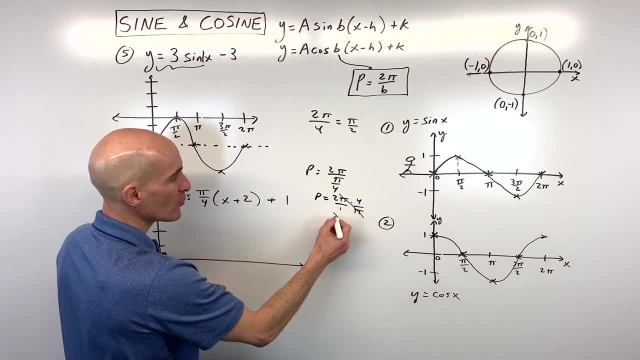 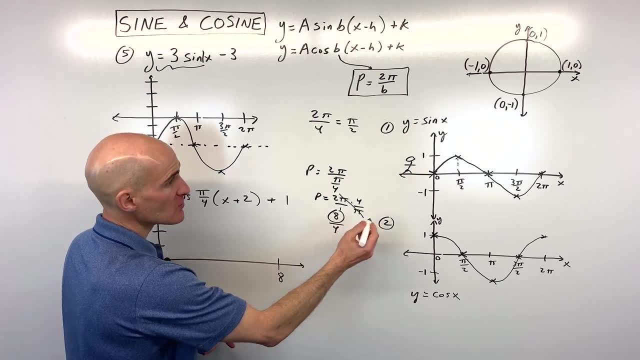 is like: 2 pi over 1. See how the pi's cancel. and 2 times 4 gives us a period of 8.. So let's go to our x-axis here. Let's call this 8.. If we divide this by 4, because, remember, we're dividing up into: 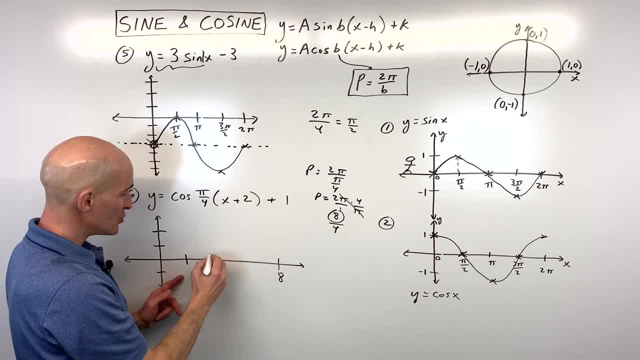 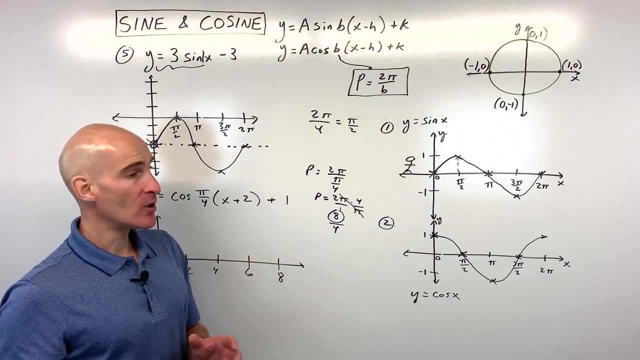 4 pieces. this is going to give us a scale of 2.. So it's going to go 2,, 4,, 6, 8.. Okay, so I just keep adding 2 each time. Now, what I like to do is: I like to take the shift into account. So this is: 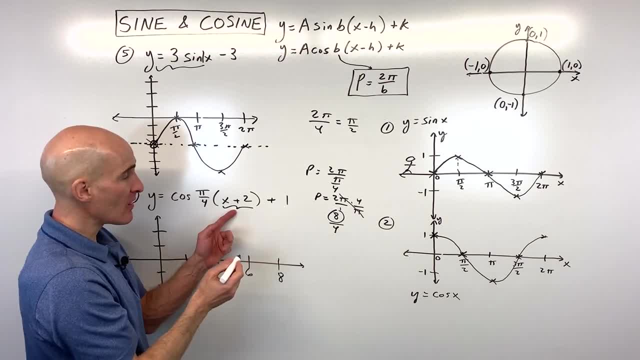 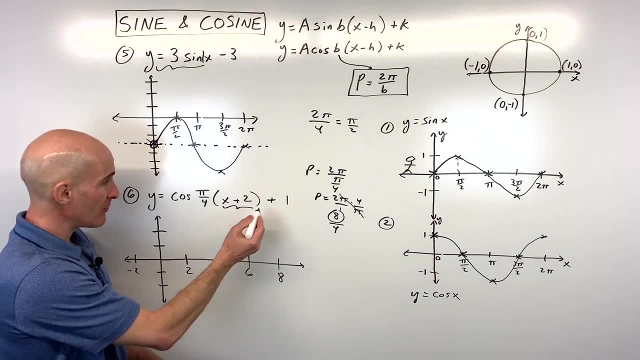 the phase shift left and right. This is our vertical shift up and down. Remember, the one group with the x has the opposite effect. So the plus 2 is actually going to shift it to the left 2, and the plus 1 is going to shift it up 1.. So what we're going to think of is going left 2,. 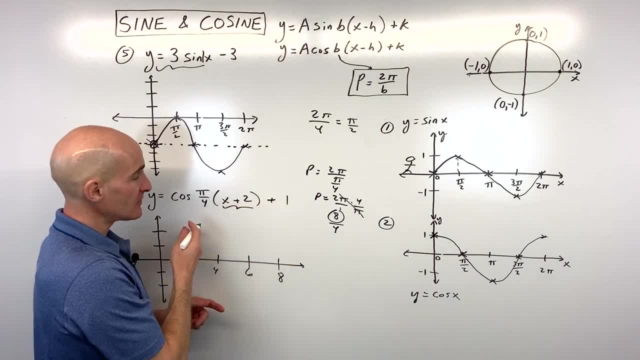 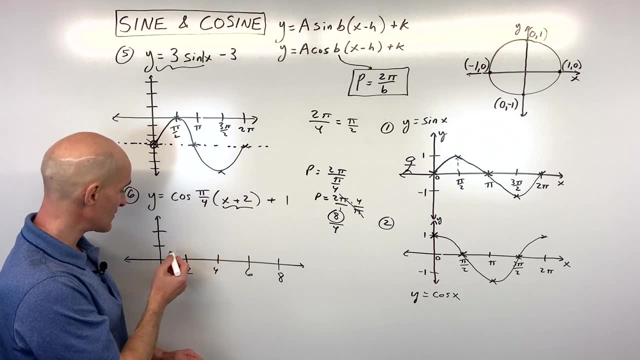 i like to take the shift into account. this is the phase shift: left and right. this is our vertical shift up and down. remember, the one group with the x has the opposite effect. so the plus two is actually going to shift it to the left two and the plus one is going to shift it up one. so what we're going to think of is going left two. 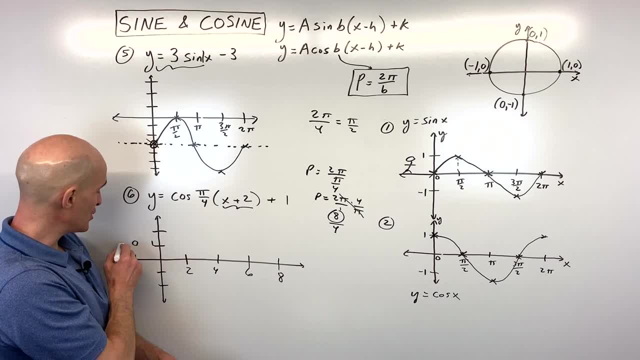 up one. this is going to be like our new starting point right here, our new origin. i like to draw in like a dashed or dotted line: okay, to represent the x-axis. you can do the same thing with the, the y-axis. so this is like our new origin. 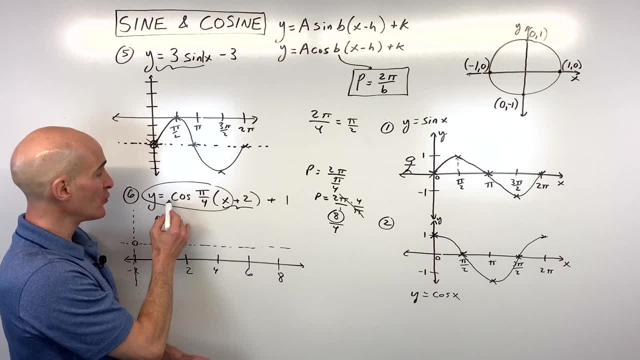 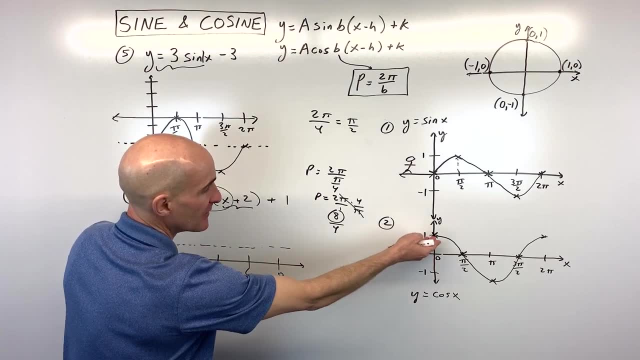 so what we're going to do is graph our cosine graph. it has an amplitude of one. see how there's nothing in front of the cosine that's understood to be one cosine, and we know that the cosine starts here, at the maximum, at the high point. so in this case, our high point is going to be at one. 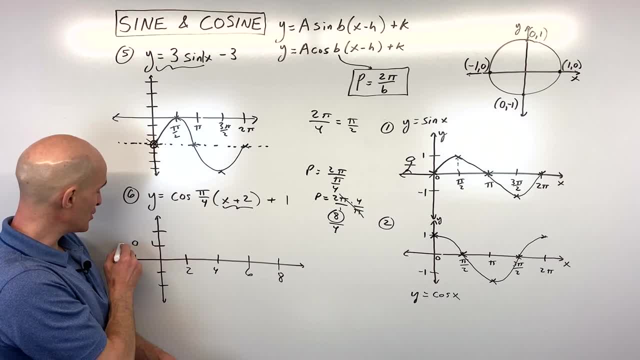 up 1. This is going to be like our new starting point right here, Our new origin. I like to draw in like a dashed or dotted line to represent the x-axis. You can do the same thing with the y-axis, So this is like our new origin. Now all we have to do is graph our 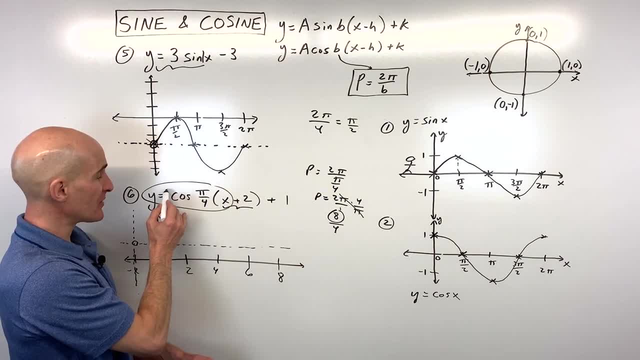 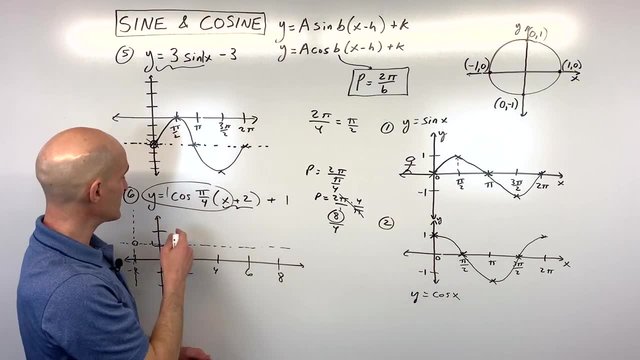 cosine graph. It has an amplitude of 1.. See how there's nothing in front of the cosine. That's understood to be 1 cosine, And we know that the cosine starts here at the maximum, at the high point. So in this case our high point is going to be at 1, because the amplitude is 1.. So it's. 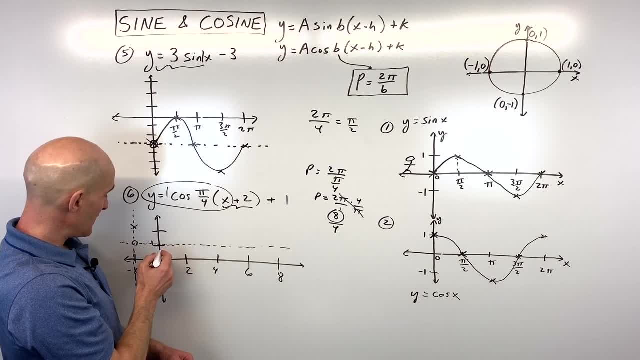 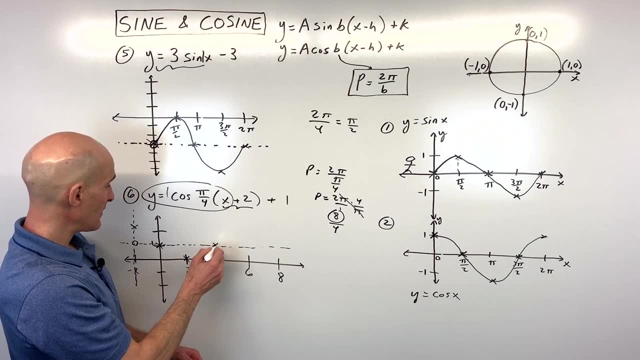 going to start here at 1.. It goes back to the 1. midline, which is going to be right here, And then it goes down to the minimum, back to the midline, and then back to the maximum, which is here at 1.. So we've got our graph. looks something like this: 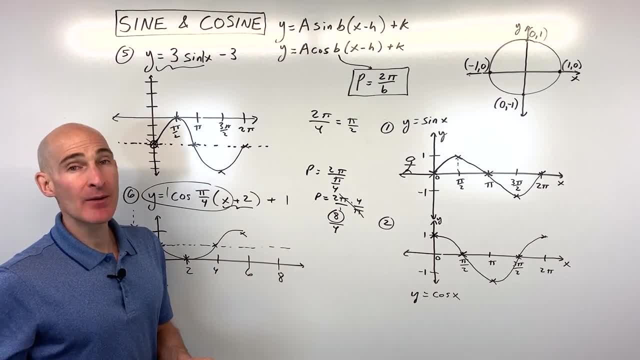 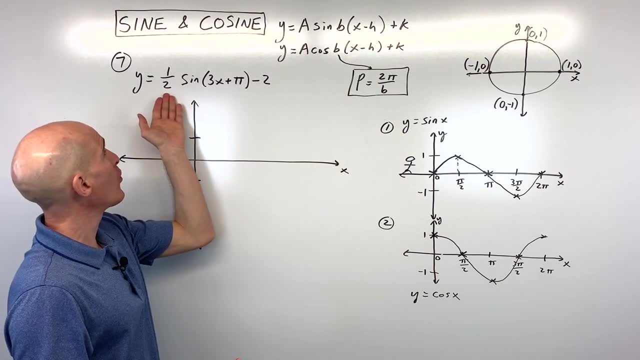 And you can keep repeating, et cetera. Let's do one last example that involves all these different transformations, so you can get a really good grasp on this. Okay, see if you can do this one. This is a real challenging example here. 1 half sine of the. 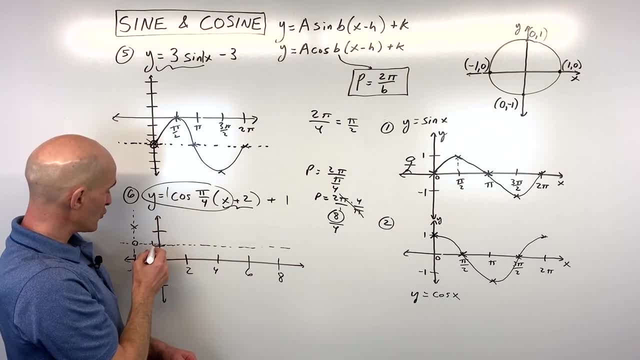 because the amplitude is one. so it's going to start here at one. it goes back to the midline, which is going to be right here, and then it goes down to the minimum, back to the midline and then back to the maximum, which is here at one. so we've got our graph. looks something like: 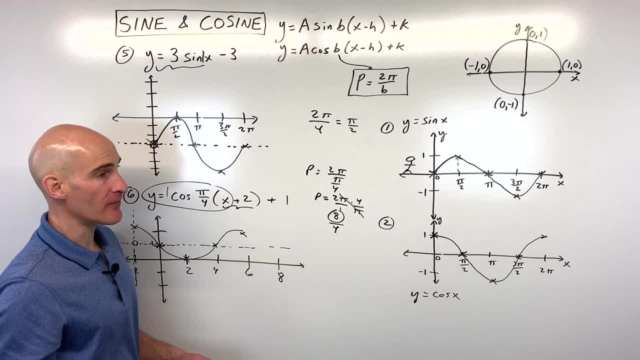 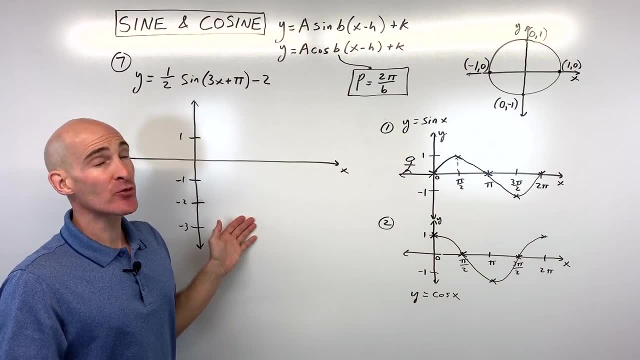 this and you can keep repeating, etc. let's do one last example that involves all these different transformations, so you can get a really good grasp on this. okay, see if you can do this one. this is a real challenging example here. one half sine of the quantity three x plus pi minus two, it's got a. 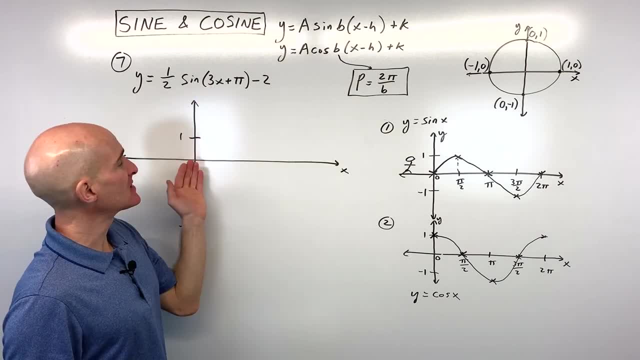 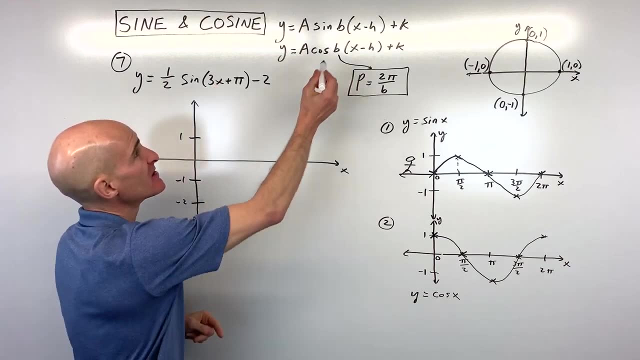 little bit of everything, and the first thing i like to do is to find that period and that x scale. so what's interesting about this problem, though, is you see how that this isn't in this form, where it's like x plus something or x minus something. 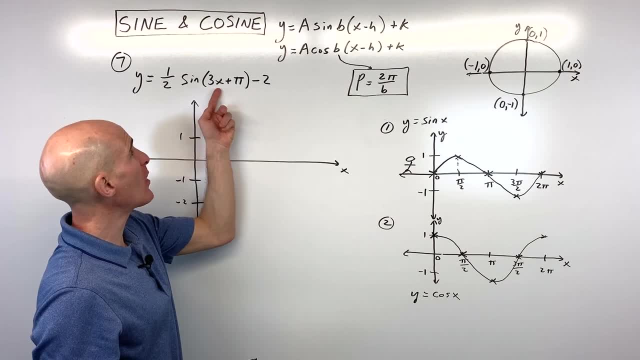 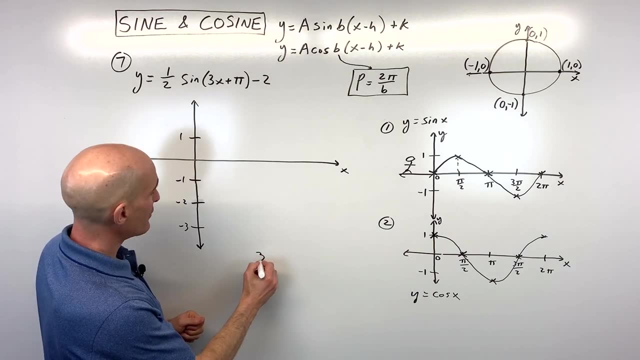 there's that three in front of the x. what we want to do is we want to factor out that three. to put it into this form, it's easier to identify the phase shift, so let's go ahead and do that. so i'm going to factor out the three, which. that's going to leave us with pi over three inside of the. 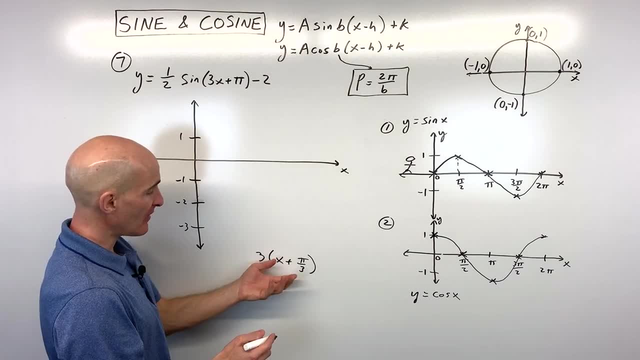 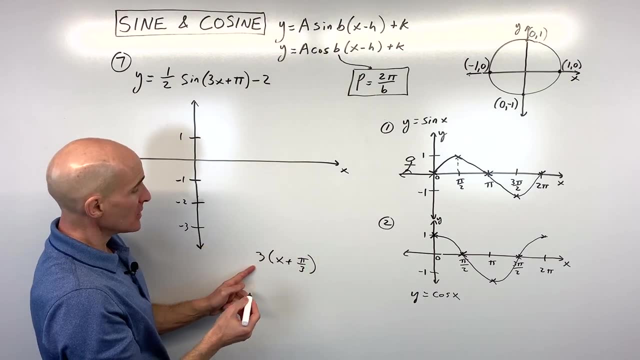 parentheses. so what i did is i, i factored out the three, or, you know, divided out the three. you can see, if you double check, by distributing you get back the three x plus pi, which is what we have here. so now you can see that that b value. 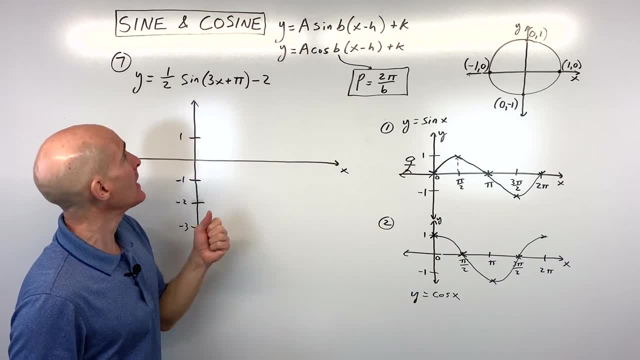 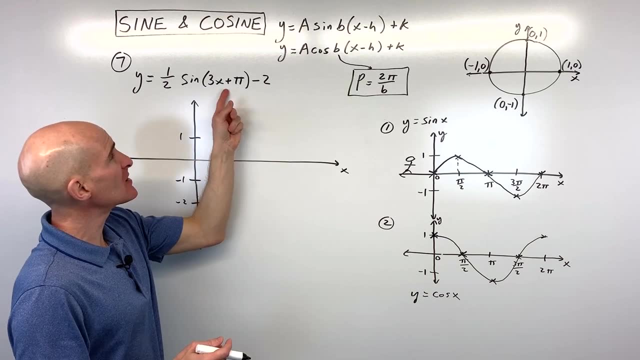 quantity 3x plus pi minus 2.. It's got a little bit of everything, And the first thing I like to do is to find that period and that x scale. So what's interesting about this problem, though, is you see how that this isn't in this form, where it's like x plus. 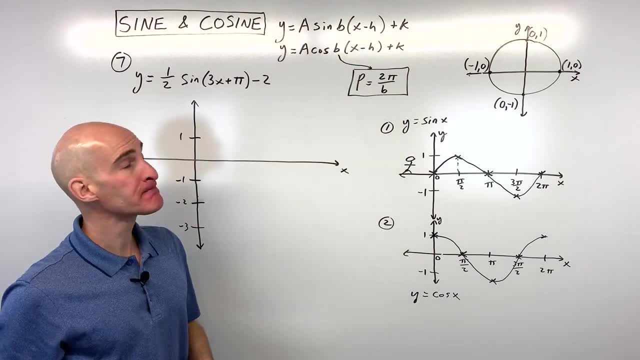 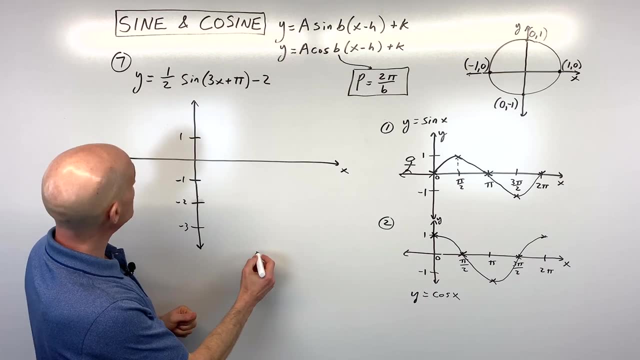 something, or x minus something. There's that 3 in front of the x. What we want to do is we want to factor out that 3. to put it into this form, it's easier to identify the phase shift. So let's go ahead and do. 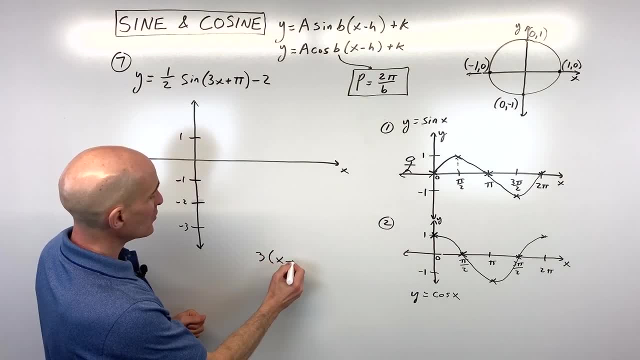 that. So I'm going to factor out the 3, which that's going to leave us with pi over 3 inside of the parentheses爲. So what I did is I put in here, let's say the minute you calculate x and minute, and I'm going to following up. let's say I'm going to calculate the suspended. 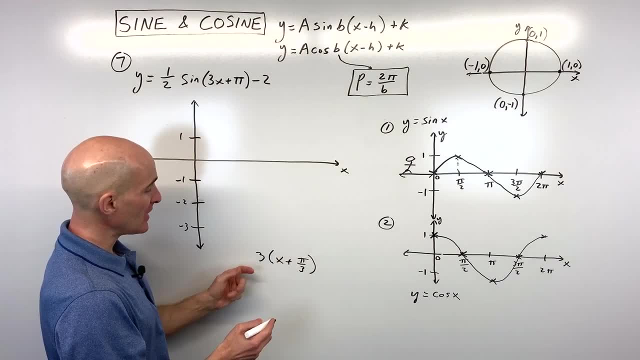 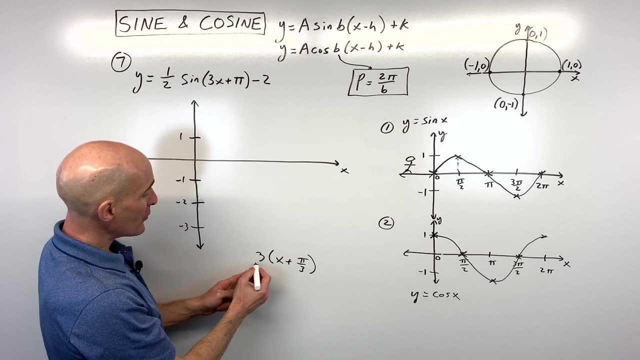 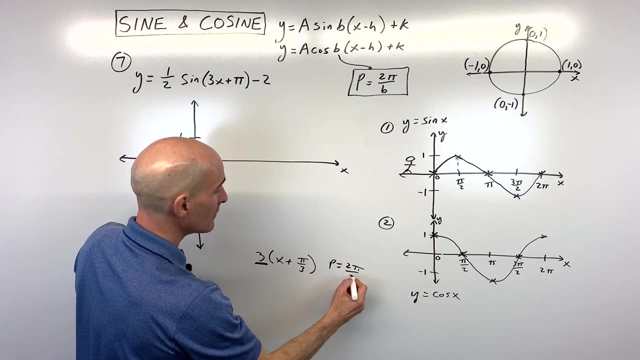 is I factored out the 3 or divided out the 3.. You can see if you double check, by distributing you get back the 3x plus pi, which is what we have here. So now you can see that that b value is 3 and our period is going to be 2 pi divided by 3.. Okay, now if we multiply, 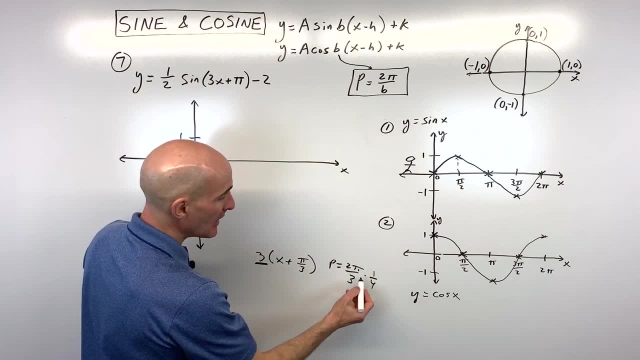 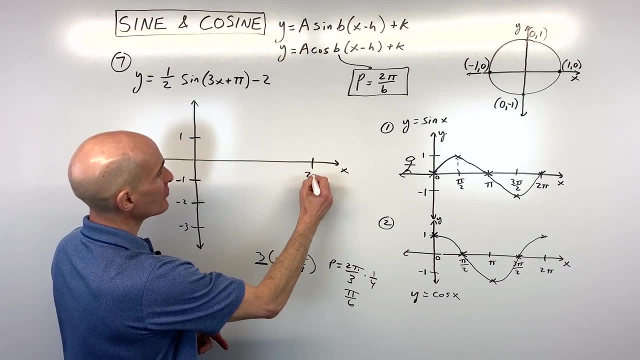 that by 1 fourth to find our scale, what we're counting by. that's going to give us 2 pi over 12, which reduces down to pi over 6.. Okay, so let's go ahead and put 2 pi over 3. 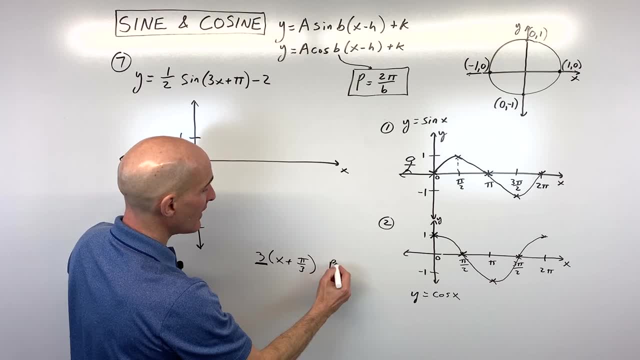 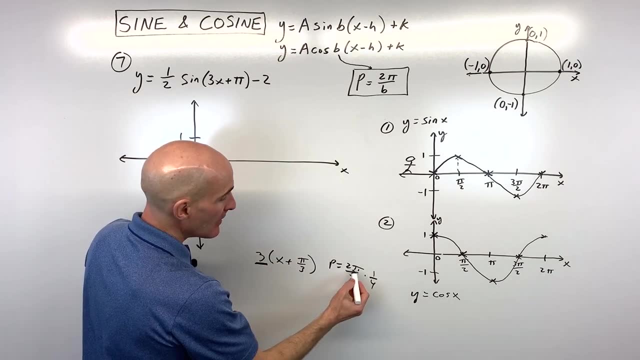 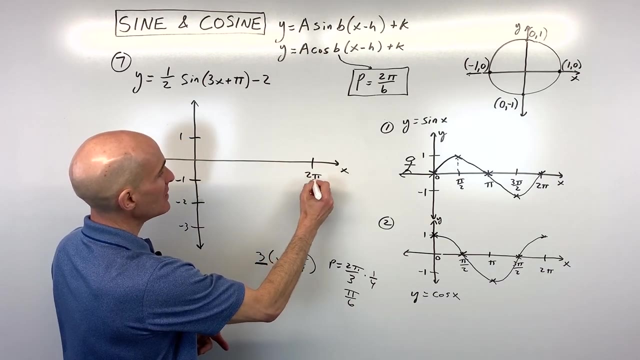 is three and our period is going to be two pi divided by three. okay, now if we multiply that by one fourth to find our scale, what we're counting by, that's going to give us two pi over twelve, which reduces down to pi over six. okay, so let's go ahead and put two pi over three here, divide that. 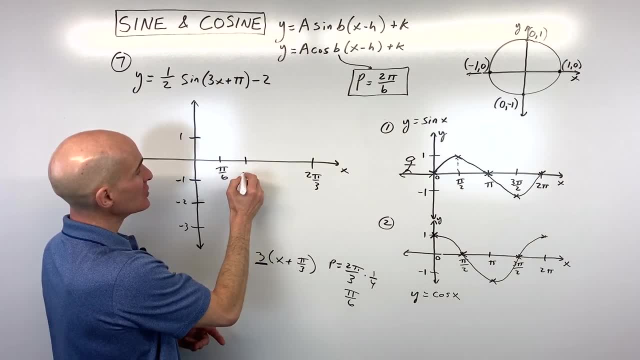 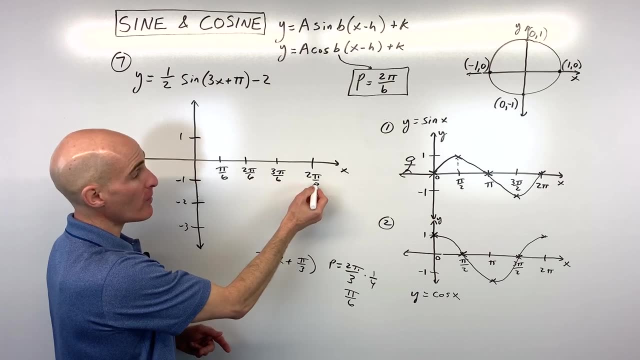 into four pieces, which is pi over six. so this is one pi over six, two pi over six. you can reduce that to pi over three, three pi over six, which is pi over two. four pi over six, which is two pi over six, two pi over three. if you go the other direction, this would be like a negative pi over six. 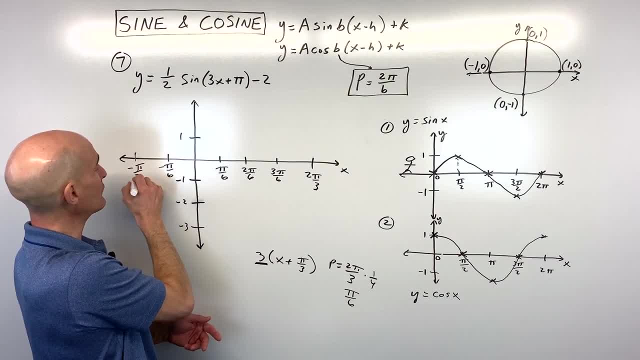 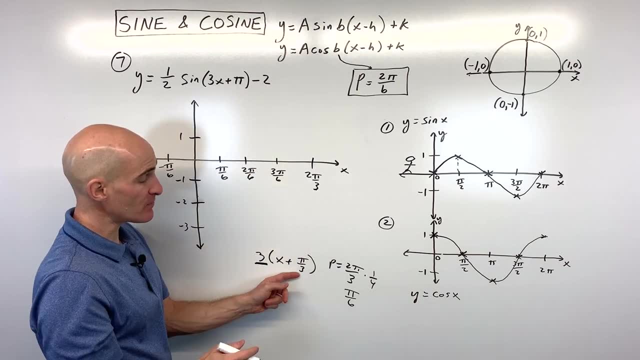 a negative two pi over six, which is a negative pi over three if you reduce. now what we want to do is we want to take into account the phase shift and the vertical shift, so the plus pi over three- remember the one group with the x has the opposite effect. this is actually. 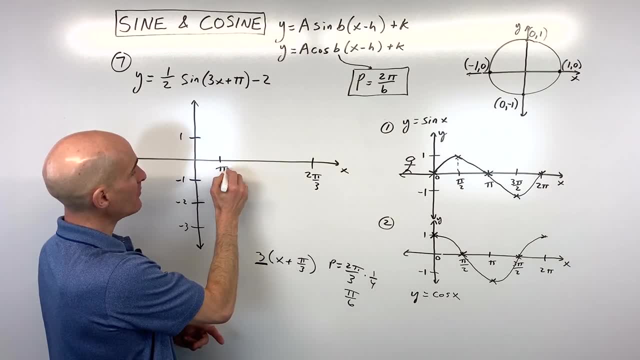 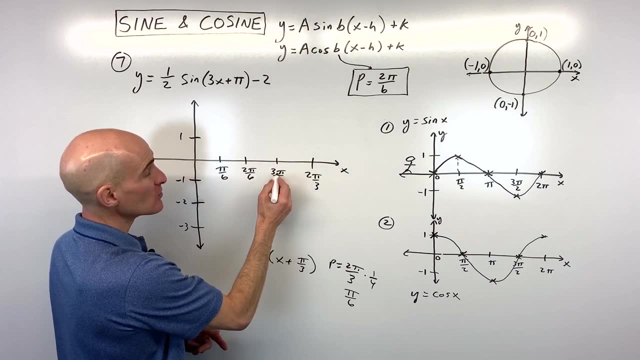 here. divide that into 4 pieces, which is pi over 6.. So this is 1 pi over 6,, 2 pi over 6, you can reduce that to pi over 3,, 3 pi over 6, which is pi over 2,, 4, pi over 6, which. 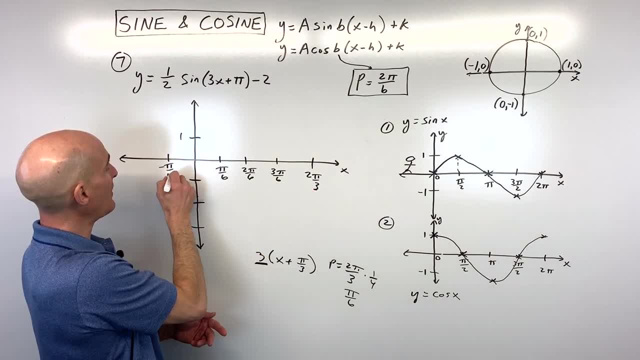 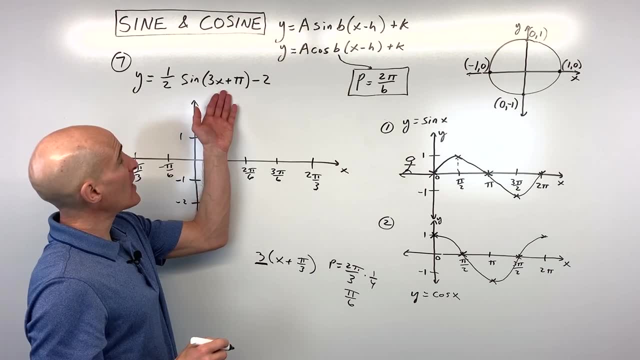 is 2 pi over 3.. If you go the other direction, this would be like a negative pi over 6, a negative 2 pi over 6, which is a negative pi over 3. if you reduce Now, what we want to do is we want to take into account the phase shift and the vertical shift, So the plus. 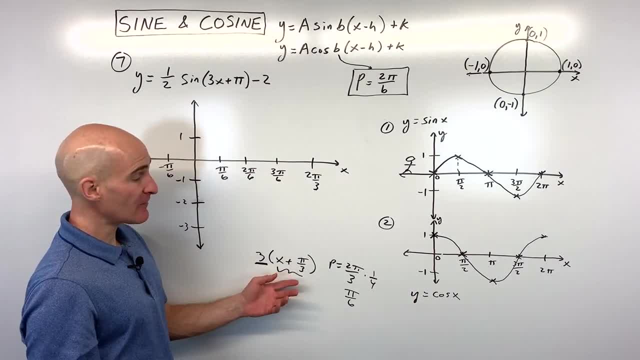 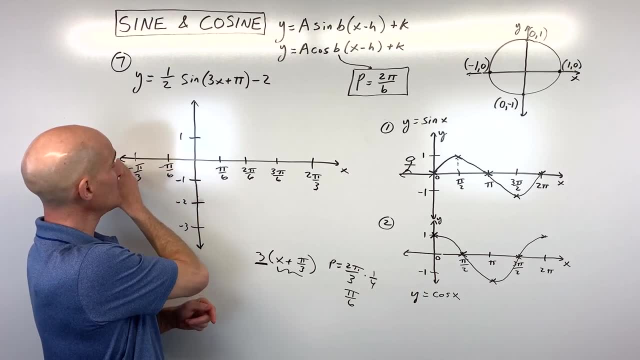 pi over 3, remember the one grouped with the x. The x has the opposite effect. This is actually going to shift to the left pi over 3.. So because our scale is pi over 6, we have to shift 2 steps to the left. So that's going to be pi. 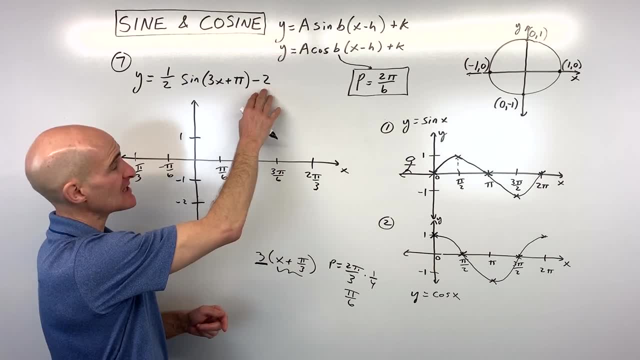 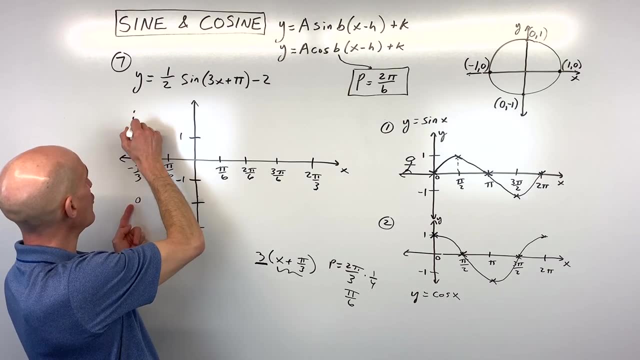 over 3, negative pi over 3. over here The minus 2 has the same effect: it's going to shift down 2.. So what I'm going to do here is I'm going to shift left pi over 3 down 2.. We're going to think of this as our new origin and you can draw in like a new axis.